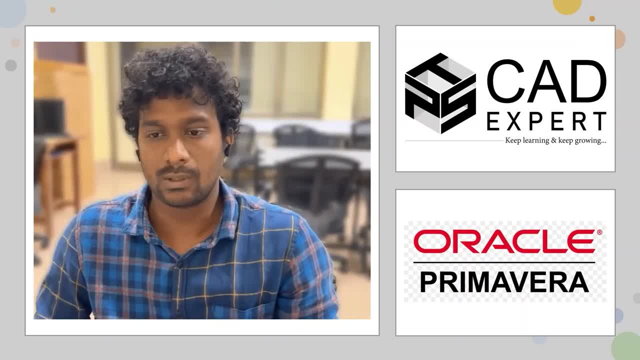 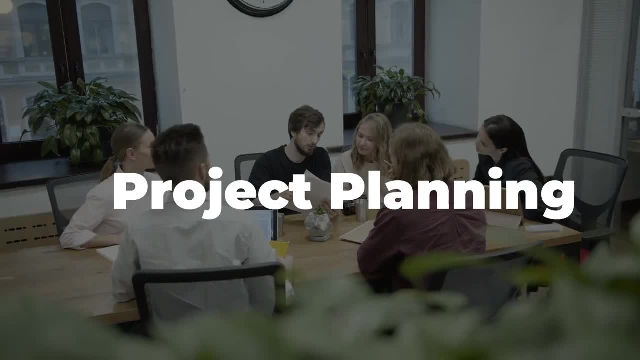 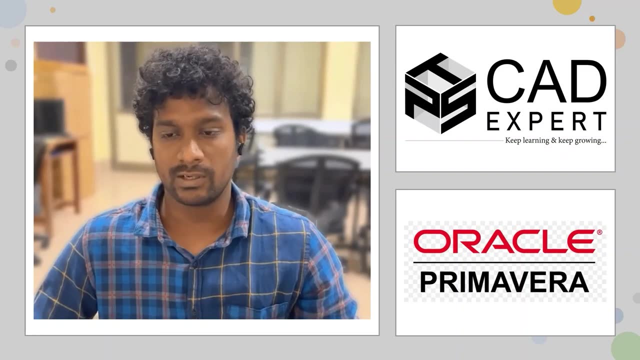 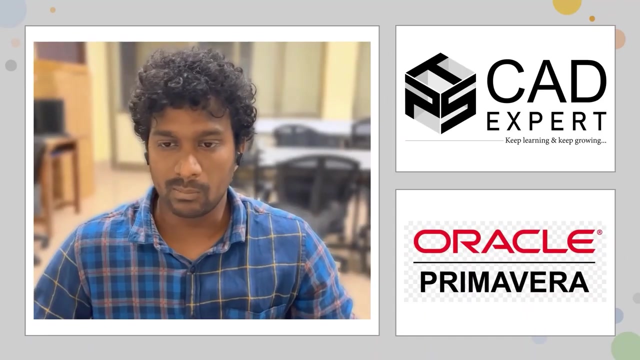 So if you look at all these issues, the majority part is coming from the management side. So there is a severe shortage skill in particularly in the project planning, The construction industry. the one skill, the one profession that has a shortage in the construction industry, the project planning. and this is the software that talks and deals with the project time and budget, the most important metrics in the project success. 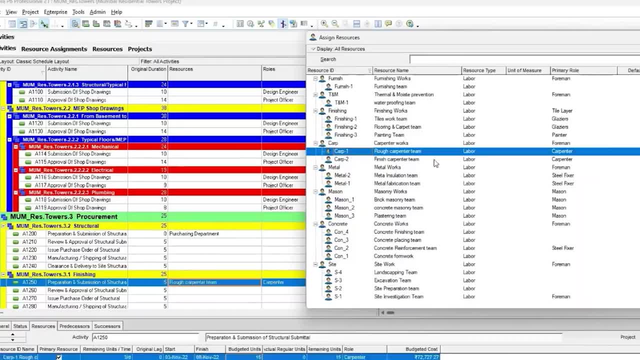 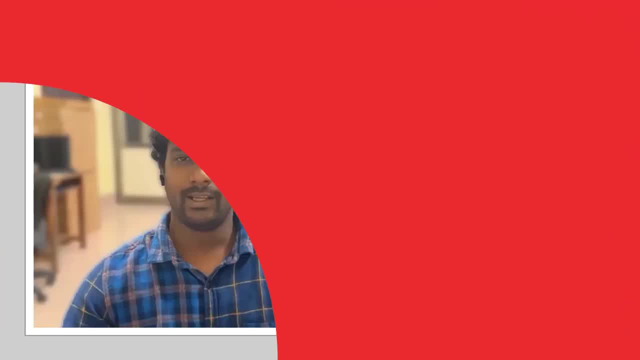 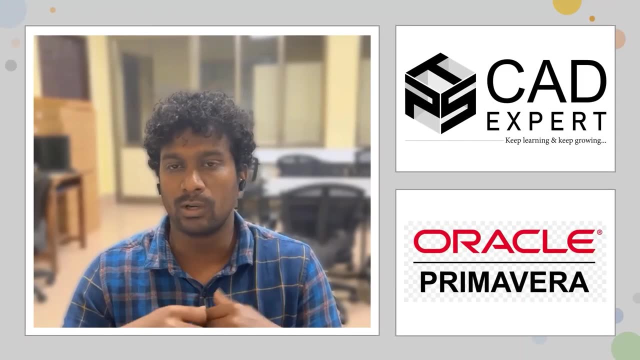 So that is the reason I'm saying the Primavera software is a much-needed skill that is required in a present construction industry And out of all project planning software, Primavera has advanced features to manage the project in program and portfolio and this makes it popular in the market, especially in UAE countries like Abu Dhabi and Dubai. 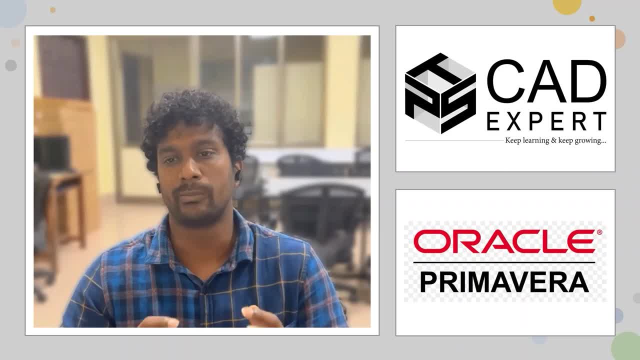 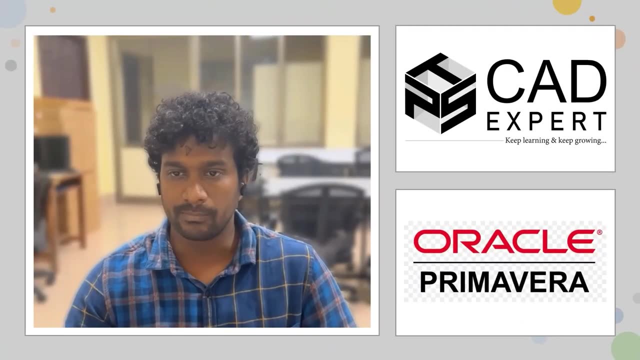 In their countries. Primavera is mandatory for every executed project. The Primavera documents used as a legal evidence in the courts when the dispute rises between the stakeholders, Because a well-executed plan gives a clear picture of how they planned and how they executed. 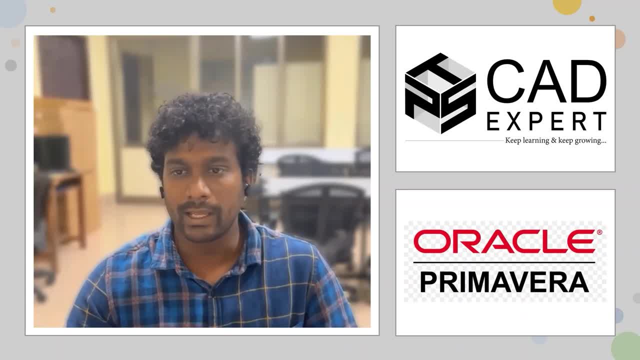 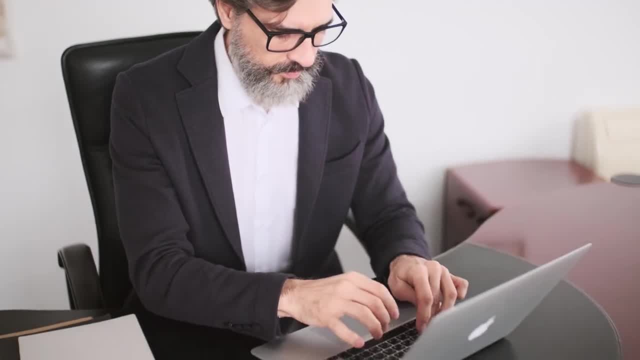 Not only in UAE. Now an Indian organization also hiring a planning engineers who have a Primavera knowledge. If you are a person, look at you as a manager position or get a job in Dubai and hence good among, This course will help you a lot. 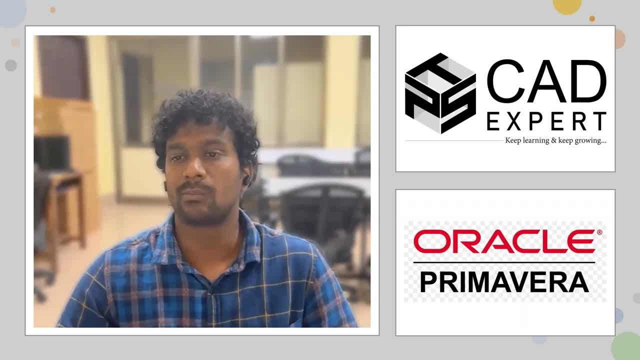 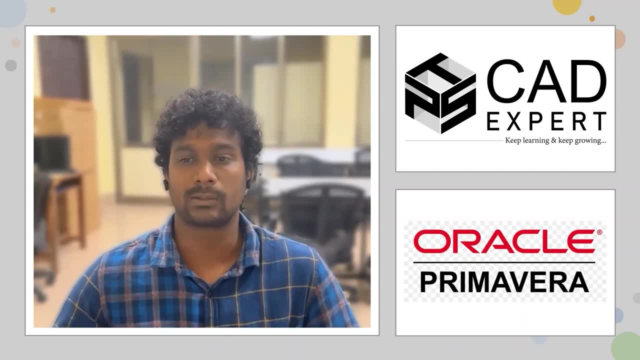 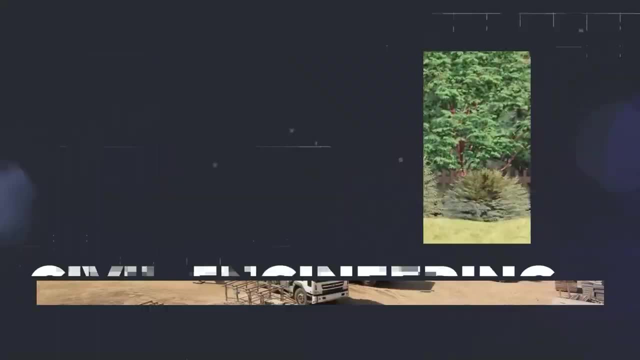 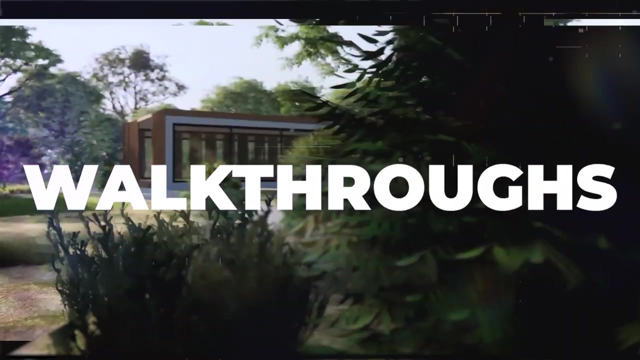 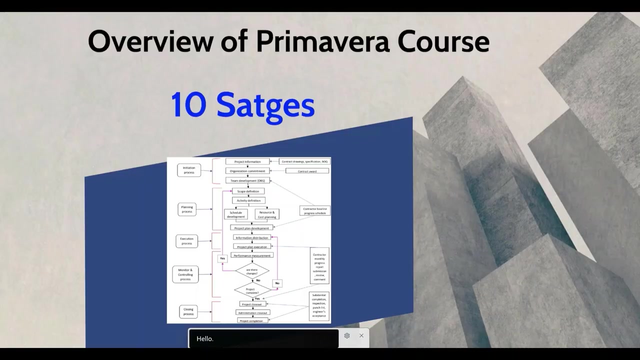 Please watch the video completely. Here you can witness some glimpse how the planning software works, how the syllabus was designed and how I am going to execute this course to expertise you in the Primavera software. Primavera software is very easy to learn. 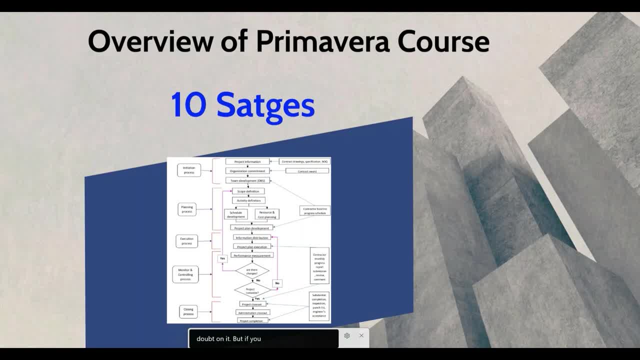 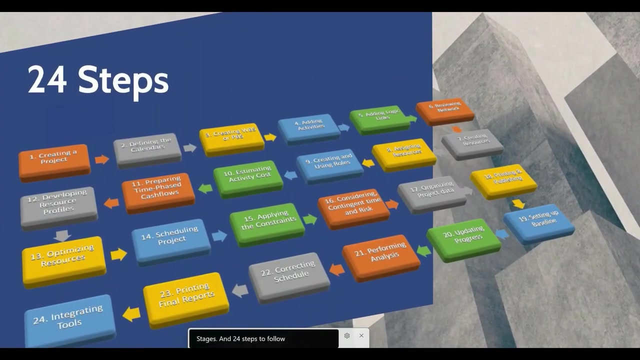 There is no doubt on it. But if you are using this software in a real-time project, it's somewhat tricky and complex process. But to get a better output from this software, We need to drive in a special direction. On a particular note, we designed this course in 10 stages and 24 steps to follow from the creating project to integrating the tools. 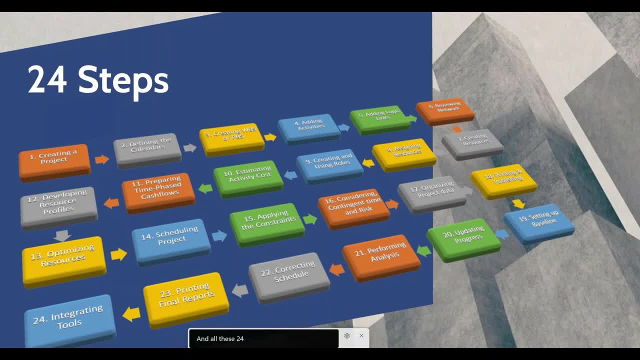 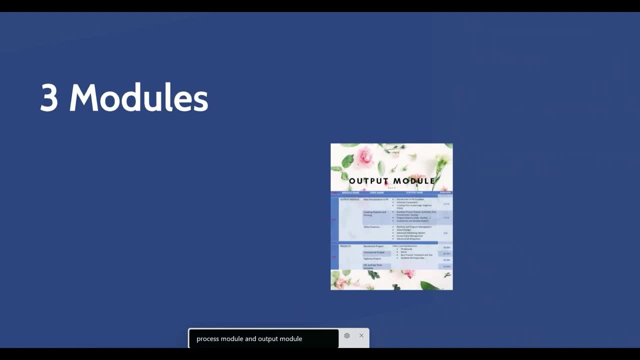 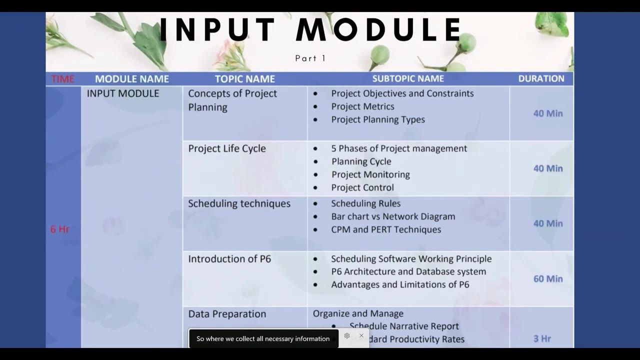 And all these 24 steps are clubbed in with three modules: One is input module, the process module and output module. Coming to input module, Where we collect all necessary information used for the scheduling and estimation of a project, This module is again divided into five chapters. 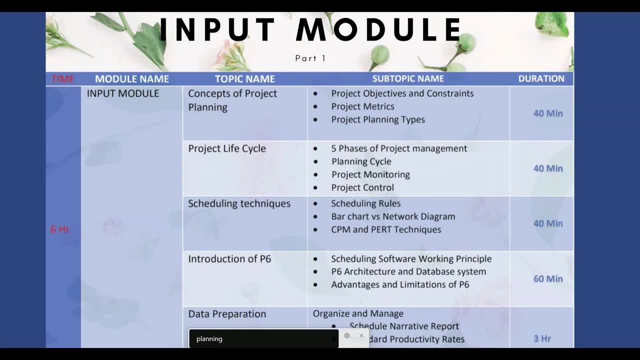 Starting from the concept of project planning, where we learn what is the project object to constraints, What are the project metrics and what are the planning types, And also the project lifecycle and project monitoring and project control. This part is a theory kind of thing. 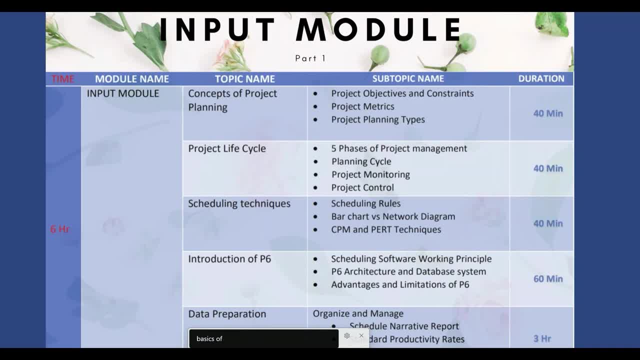 Where we learn the basics of a project planning. Then we learn the scheduling techniques, The bar chart, network diagram and CPM method. So this CPM method is the method used in the Primavera software, And then the little introduction about Primavera P6 software. 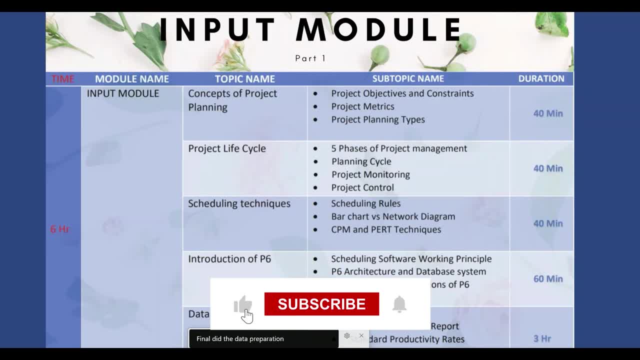 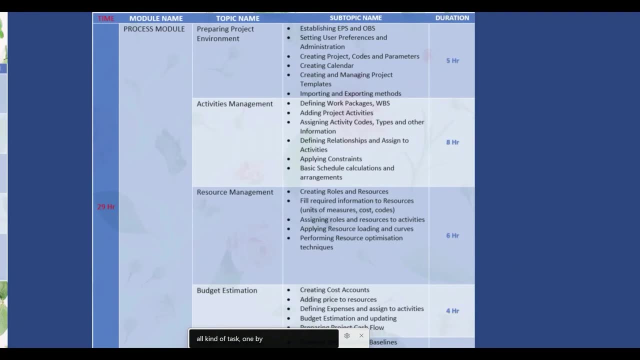 And the final data preparation. So we required some data to fill during the execution of the software, In the process module, where we all perform all kind of tasks one by one And also we fill the data when it is required. This is the process module. 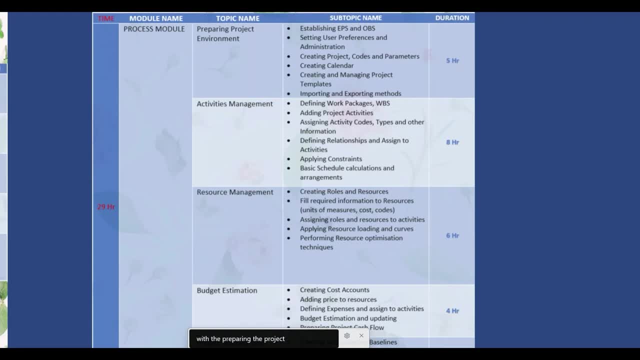 First we start with the preparing the project environment by establishing the enterprise project structure, Organization, breaking structure And creating manage project templates and all these things in the first chapter. And then that's it, And then the activities management. Here we define the work packages. 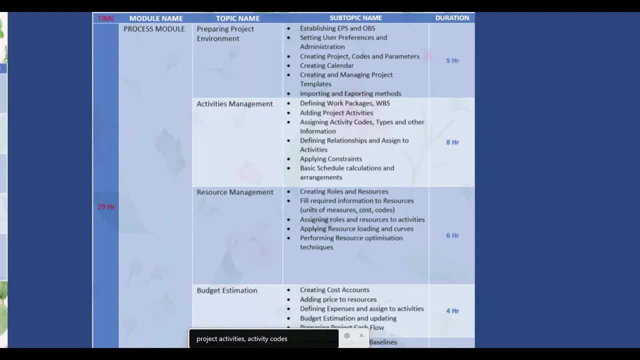 Adding the project activities, Assigning the activity codes And giving relationship to the activities And assigning the resources and everything And coming. the third chapter is like resource management, Where we create all kind of roles and the resources that is required to complete the activities. 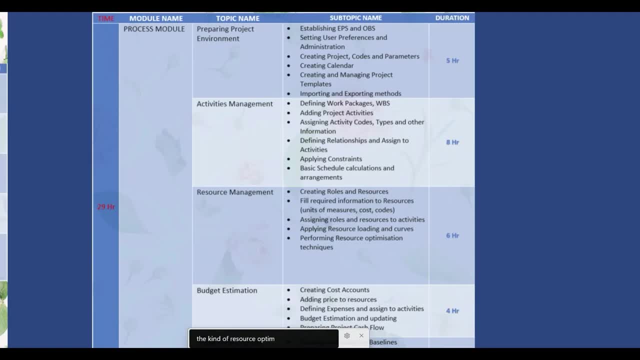 And also we perform the kind of resource optimization techniques. And the fourth chapter in the process module is the budget estimation, Creating the cost accounts, Adding the price to the resources and everything. And finally we update the progress in the fifth chapter in the process module. 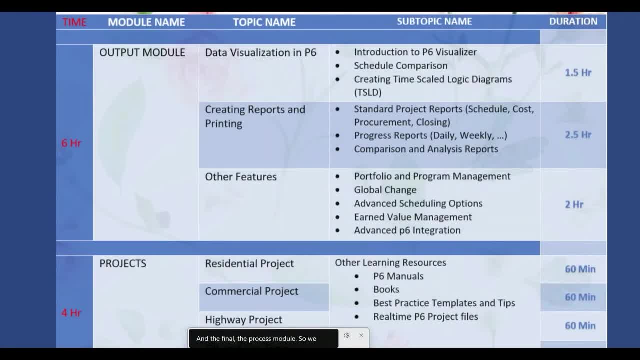 The final, the process module. So we done all kind of works in the process module. In the output module we will get different kinds of reports That are required, The standard reports that are required in the project execution. So for this purpose we use some kind of data visualization tool. 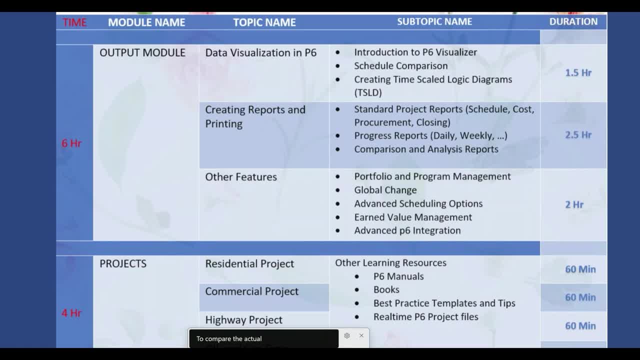 To compare the actual to budgeted, planned versus actual And also progress reports, Comparison and analysis reports And also additional features we discuss in the output module: The portfolio organizing of programs And organizing of projects in a portfolio or program management And advanced scheduling techniques options. 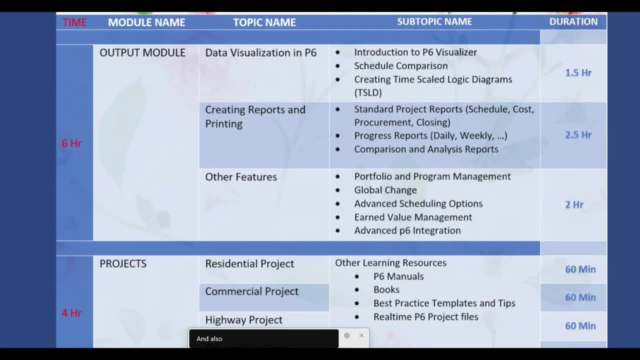 And value management, And also advanced P6 integration with different tools. At the end, we perform the four different kind of projects- Real time projects- And also we will provide you the P6 manuals and books And, more importantly, best practice to use this software in a correct manner. 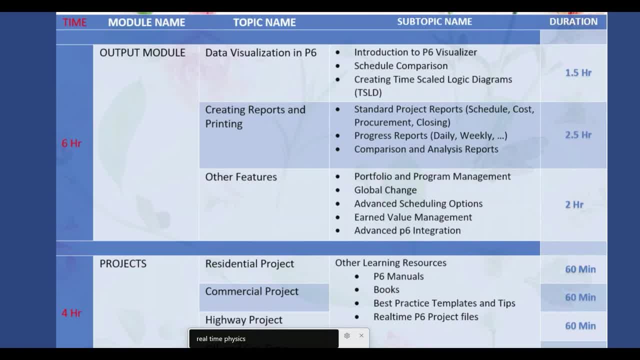 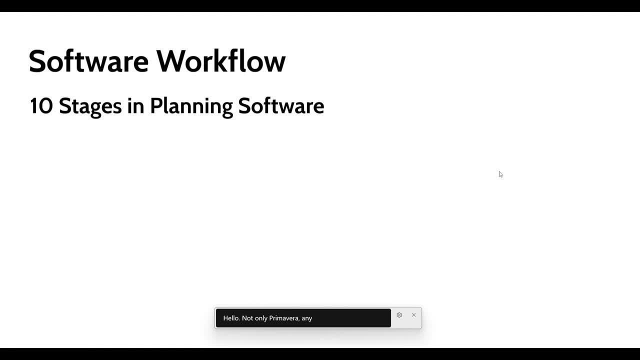 And also you will get a real time P6 project files at the end. Not only Primavera, Any kind of software have set up rules in the process. This process we call workflow of a software. So there are ten stages in the Primavera software. 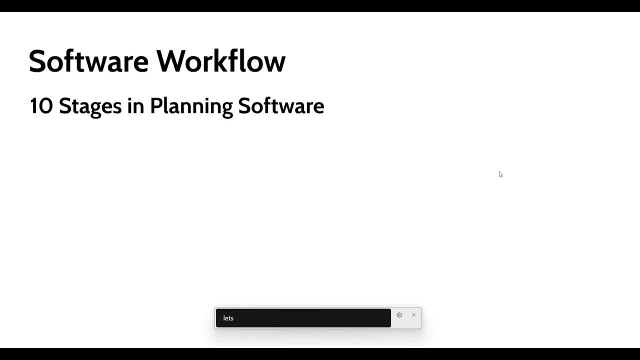 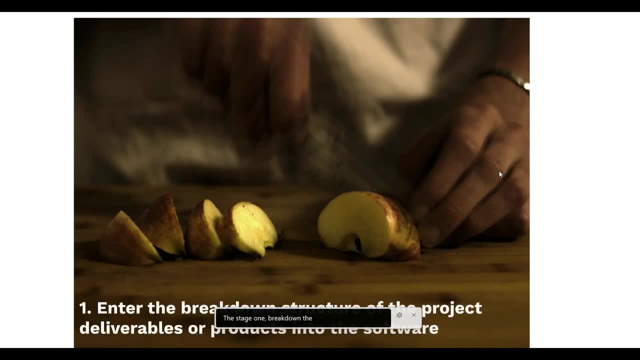 In its workflow. So let's discuss one by one The stage one. Break down the project into a measurable pieces, Like how we cut the apple into pieces to easily have it. So at the end of the day We will have a work breakdown structure of your entire project. 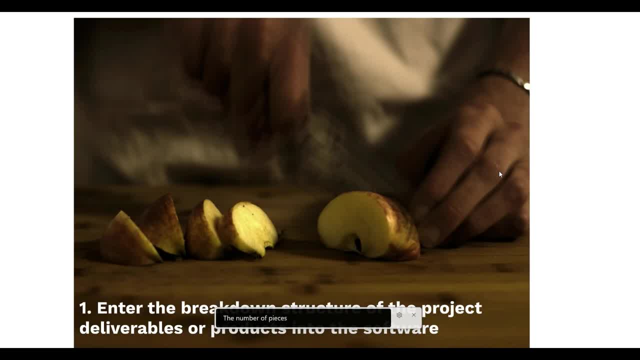 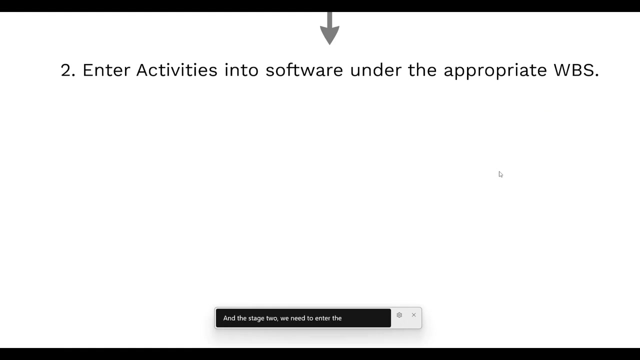 The number of pieces and the number of parts will depends upon the type of the project and size of the project. If your project is a beginner, So you must have a lot of work breakdown in your project And the stage two. We need to enter the activities into each work breakdown. 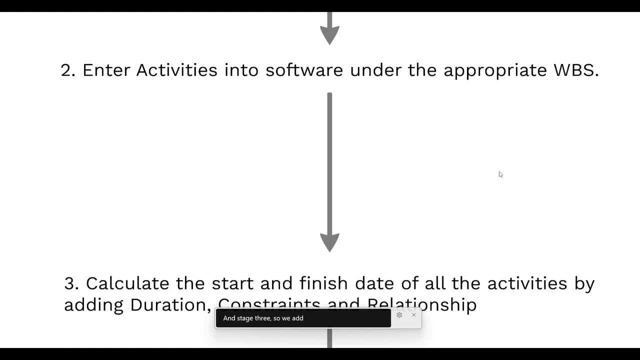 The stage three. So we add the information like duration constraints, to each and every activity And connect all these activities with one another in a closed network. So at the end of the day You will get the start and finish date of every activity. 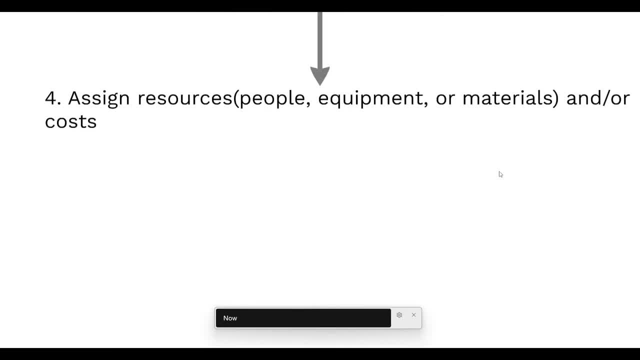 Now in the stage number four, We assign resources like people, material and equipment to the activities And you get you know cost of each activity by assigning resources, with the cost information And also you will get the budget of your project, The budget of your entire project. 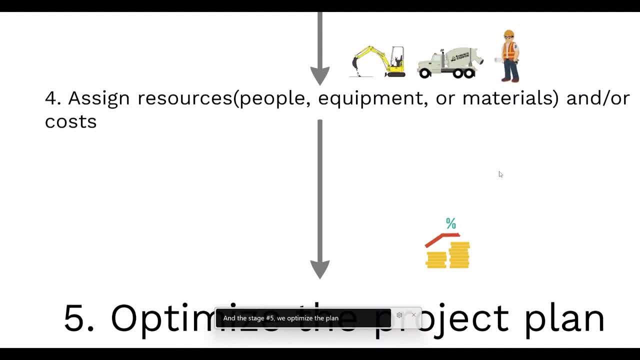 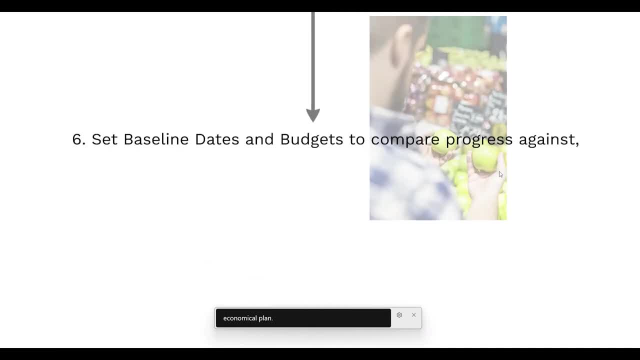 In the stage number five, We optimize the plan and project the dates, the budget and come with a practical and economical plan And set the baseline dates and budget to compare the progress. So when you're going for execution, So we need a baseline set and budget. 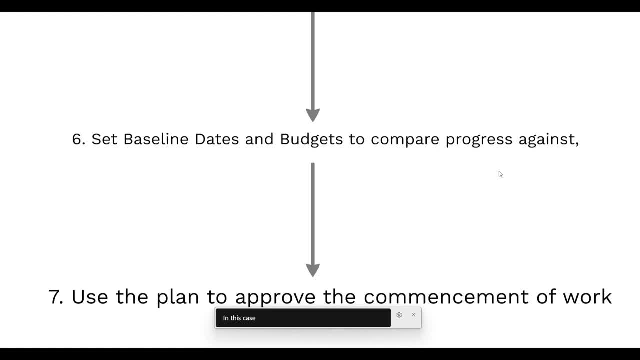 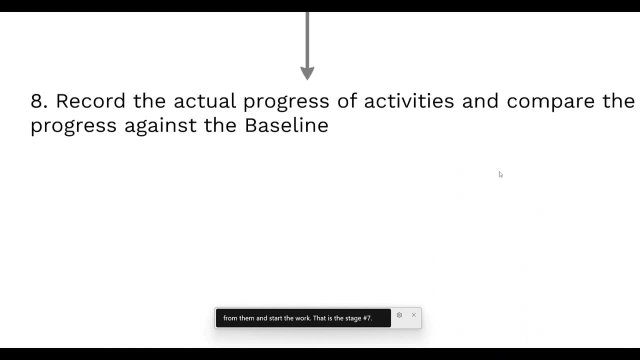 The stage seven To well document the plan and communicate with all the stakeholders And get a proof from them And start the work. That is the stage number seven And in this phase, number eight, We just record the actual progress of activities. 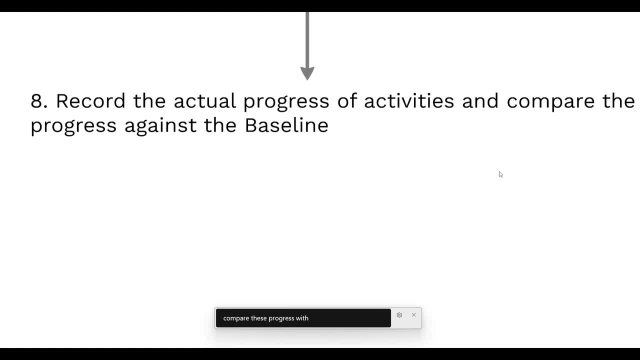 And compare this progress with the against the baseline That we already fixed in the stage number six. And then we record the final progress That we already fixed in the stage number five. In the stage nine, not only the progress, We also record the consumption of resources. 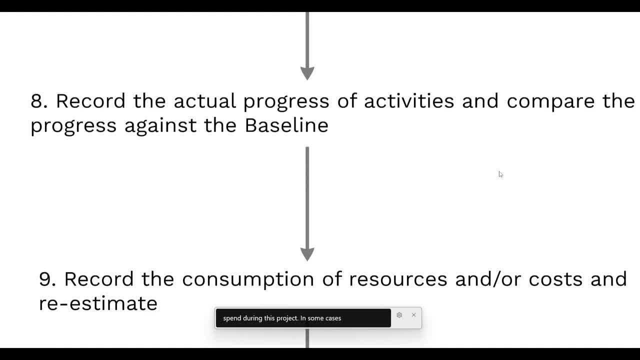 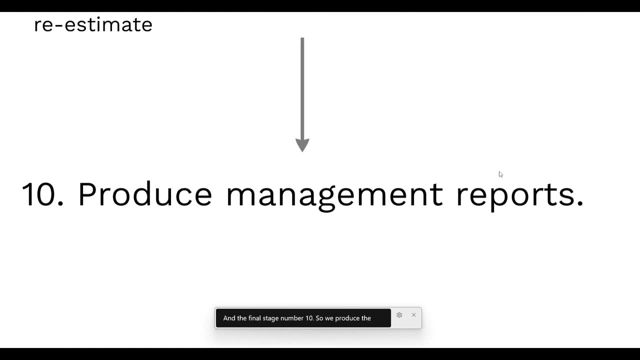 And the money that you spend during this project. In some cases we need to reestimate the resources And we need to add extra resources And extra money is required to finish the entire project. the final stage, number 10, so we produce the management reports. 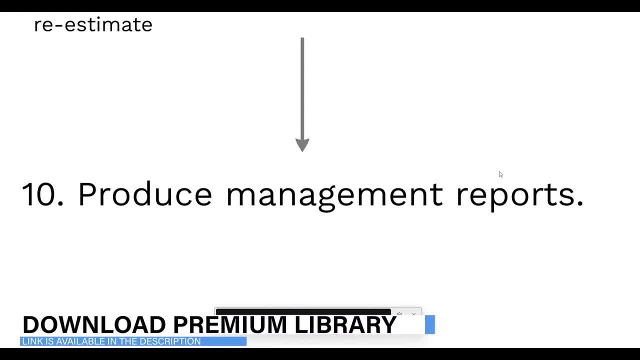 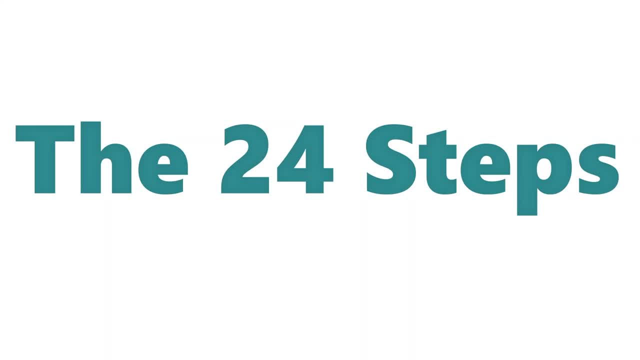 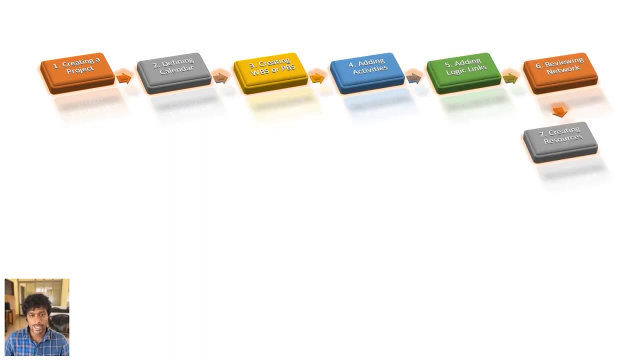 these reports used for the closing the project and also we need to- we need to send these documents to the client. as i mentioned earlier, this primary course is designed in 24 steps, from creating a project to the printing of final reports and integrating with other tools, so we execute all these 24 steps. 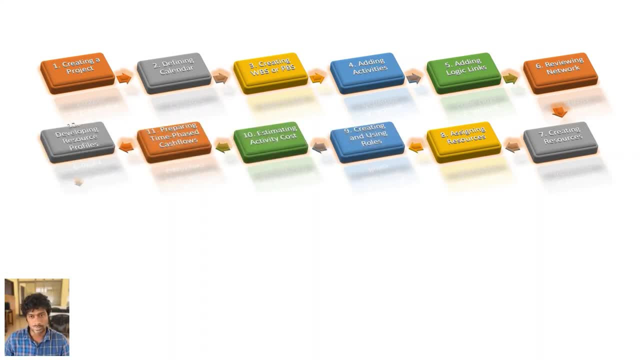 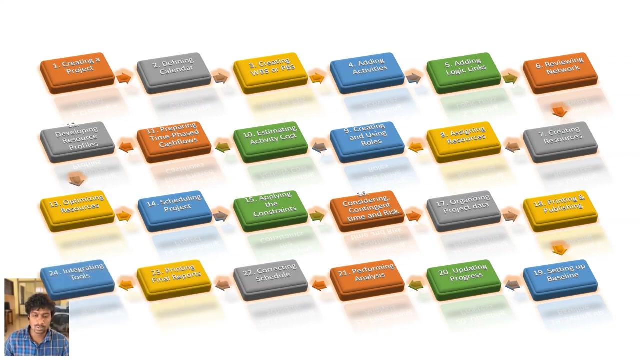 in the process module and output module in our syllabus. so by spending around 24 hours, and whereas in input module i will give you about basic concepts that will help you to understand the entire process in the primary. so let's explore the each and every steps in one by one. 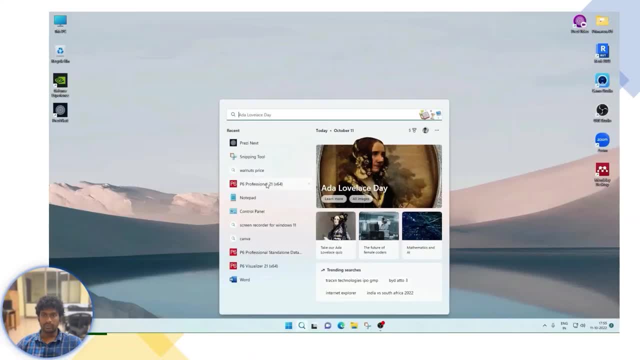 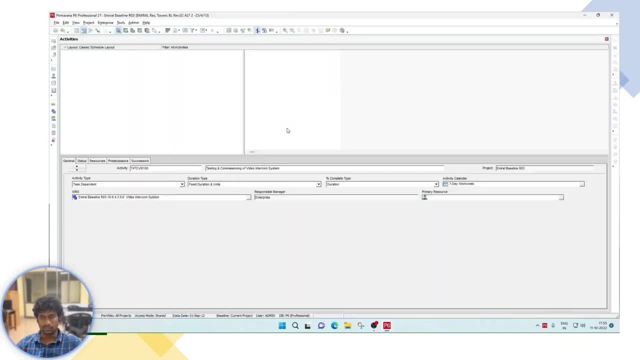 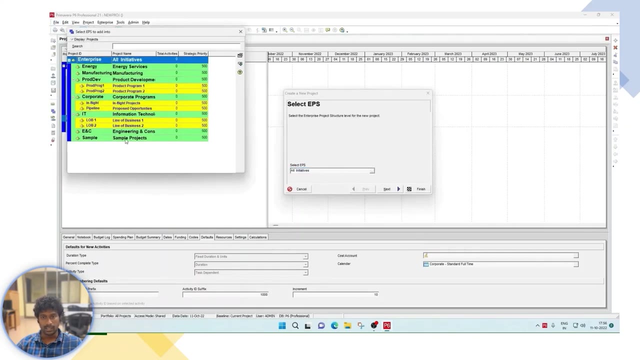 let's start with the first step, which is creating a project. once you log in the software, the first job is to create a project with the relevant information based on type of project. you need to select appropriate eps node and then you need to enter project unique id, the project name, when the project is starting and who. 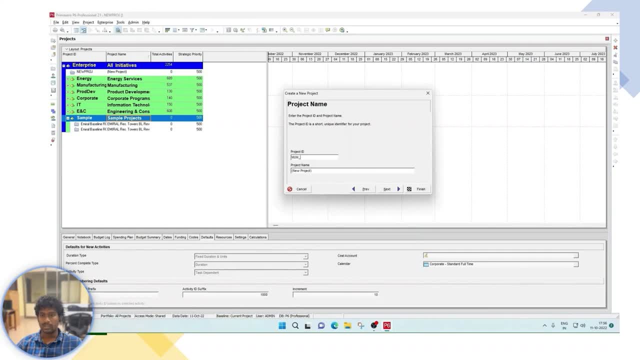 is the responsible for the project. other information like location and contact details- these are optional- you can store in the project nodes if eps node or obs node are available. it's our job to create a project based on the relevant information and then you need to enter project. 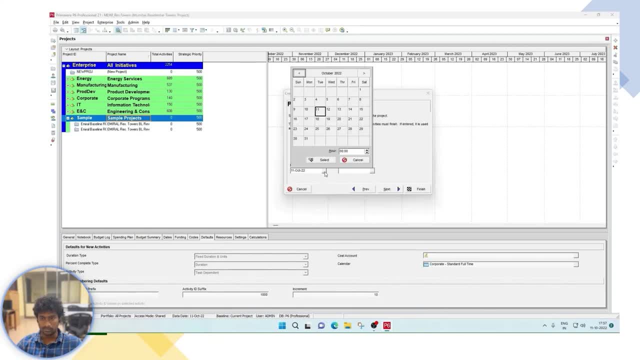 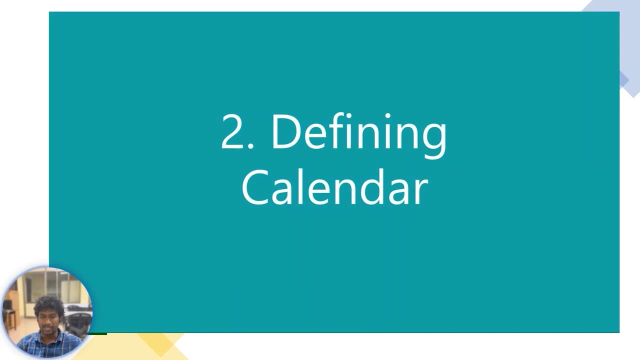 into the software before project creation. so once you create the project, then the next task is like. step two is defining a calendars. so before adding activities into your schedule, it is important to define the calendar. defining a calendar means defining a working hours in a day and working. 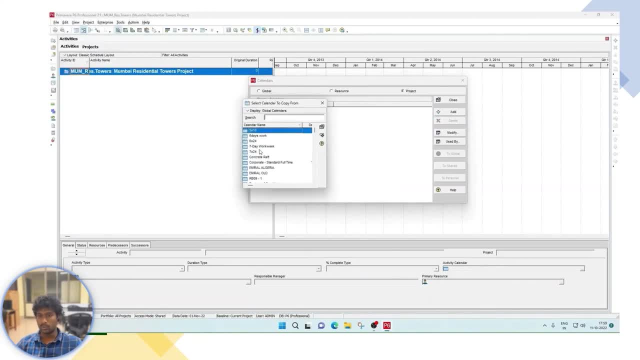 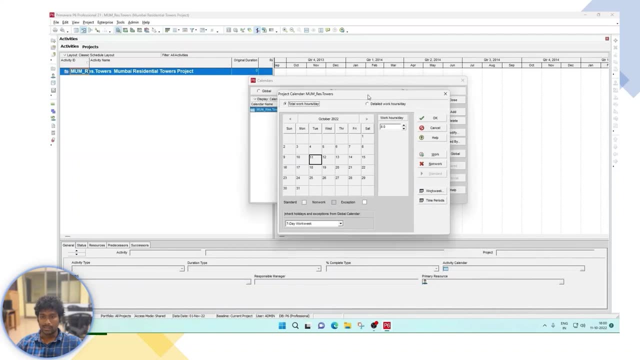 days in a year. this calendars plays important role in your time calculations in the primavera software. primavera has three types of calendars. one is global calendar. you can assign any project or resource to these calendars. so these calendars are managed by in enterprise level. so another 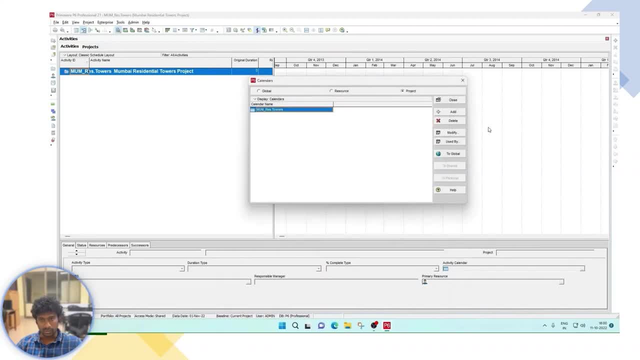 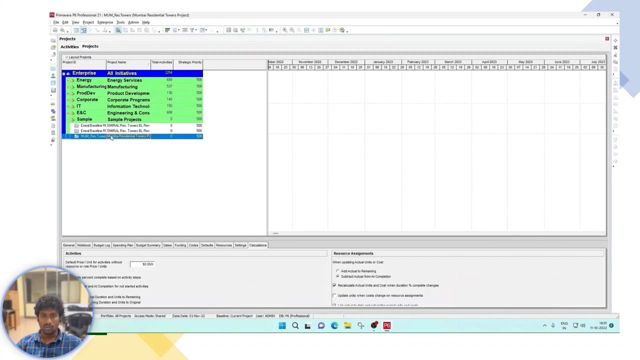 one is project specific calendars. only a particular project follows a working hours and working days stored in a project calendar. another one is resource calendar is the same as the project calendar. it's dedicated for the resources. so some resource, like heavy missionary, works only in a particular hours in a particular days once. once you're done the calendar, next job. 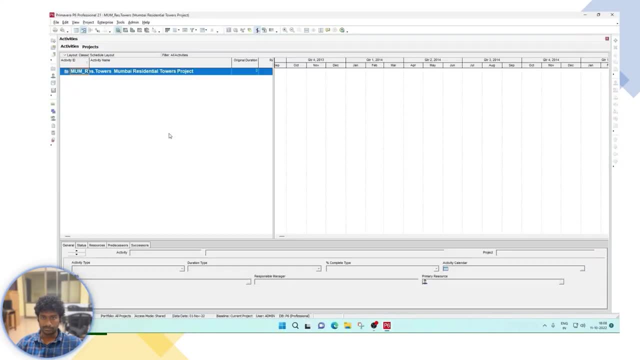 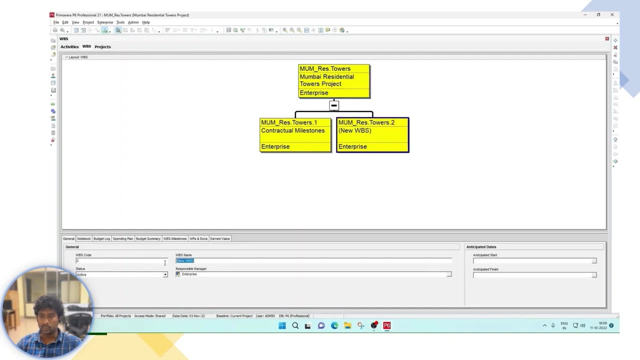 is creating a wbs and project breakdown structure. it is the breakdown of a project into a smaller component. the wbs means the structure of project into a manageable deliverables so each deliverable of can be further broken into a subtask. so the number of components that depends upon the 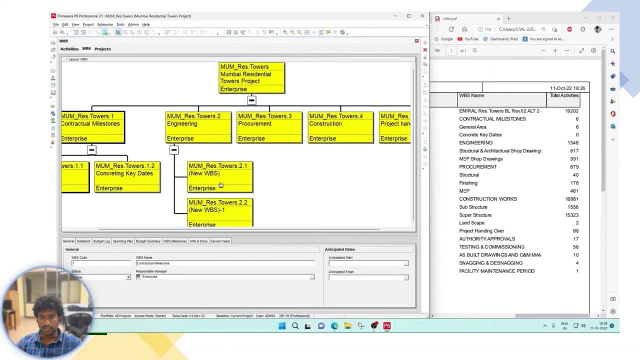 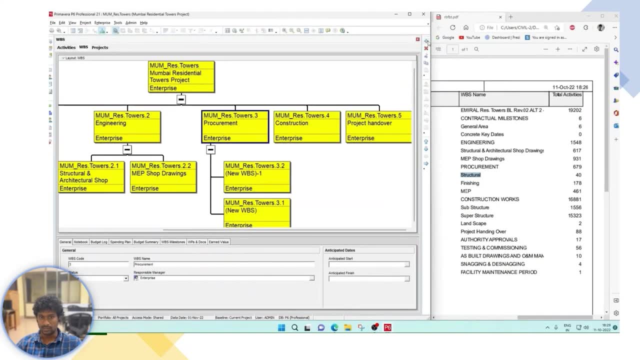 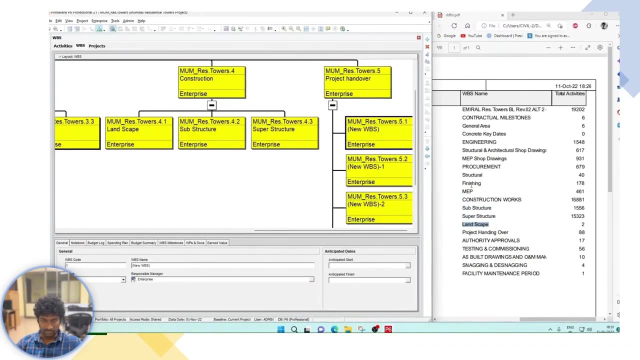 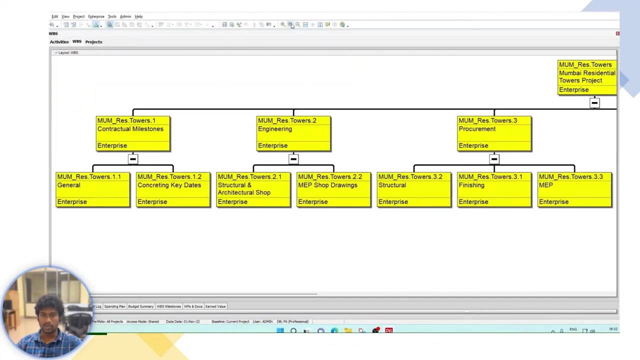 type of project. okay, that type of departments are involved. type of disciplines are involved in the project. there is no specific and mandatory formula for this, so usually reading we decompose the project based on the phases: the design phase, the procurement phase, and construction phase and closing phase. so once you complete the breakdown, the next job is adding activities. 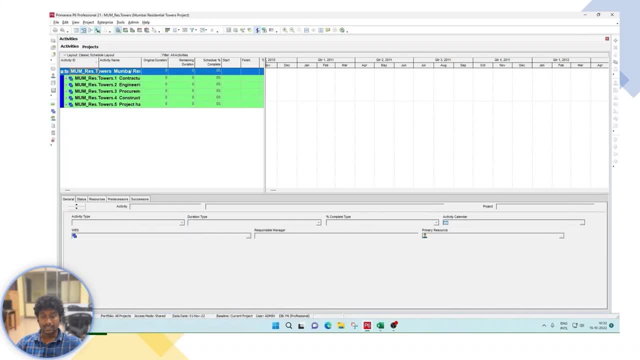 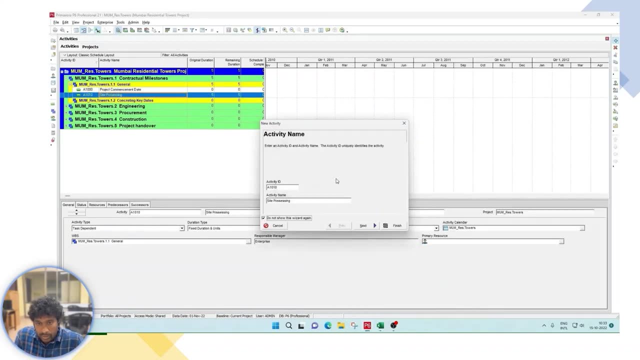 into the each component. these are the smallest parts in your project, so the first part is the project breakdown structure. the p6 works on the concept of activity, so it is very important to understand how the how the activity works in a project management activity is defined as the amount of work you perform. that converts the 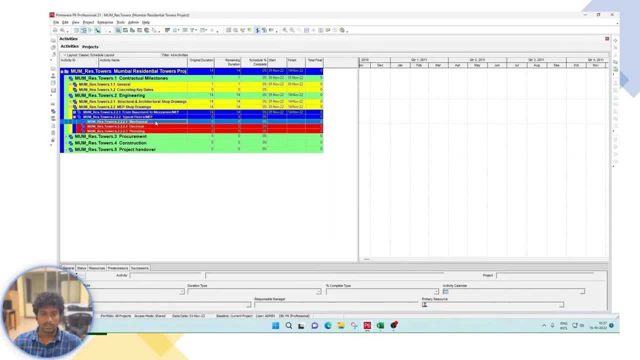 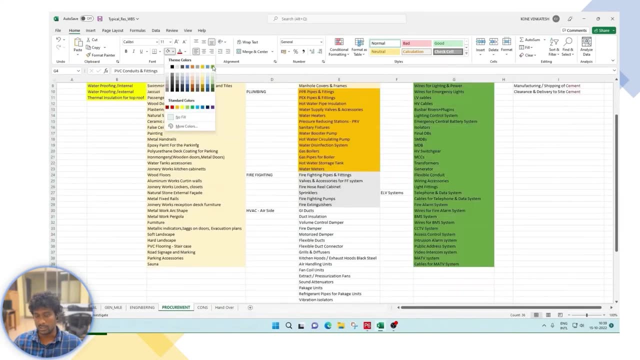 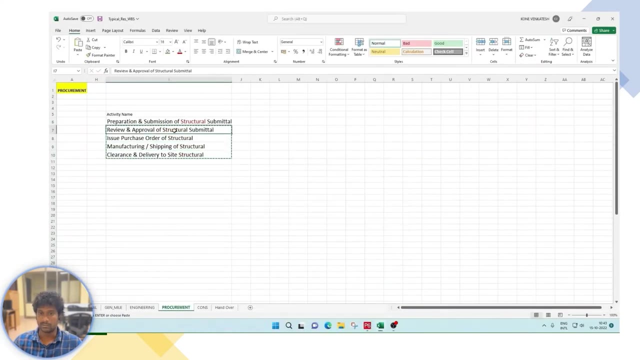 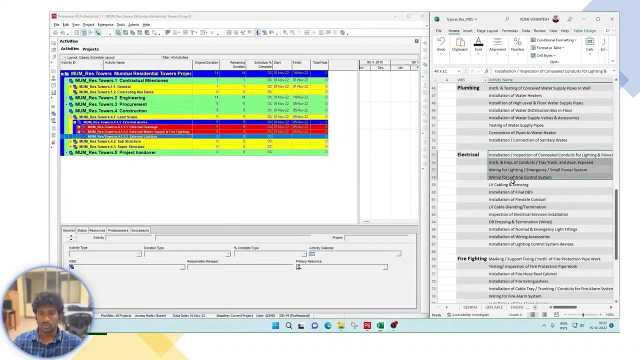 raw materials, the resources, into a deliverable product. but suppose, constructing a column, we need to perform some kind of activities, like the farm work, reinforcement and placing concrete in the pumps, concrete pumps and curing with the water. okay, these are the activities, okay, that are used to construct a column. likewise, the concept is very simple, so we need to add all required. 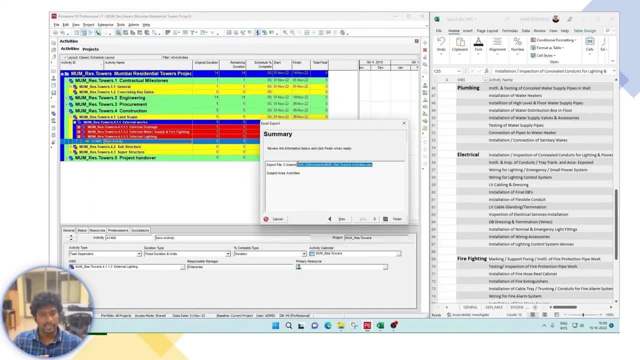 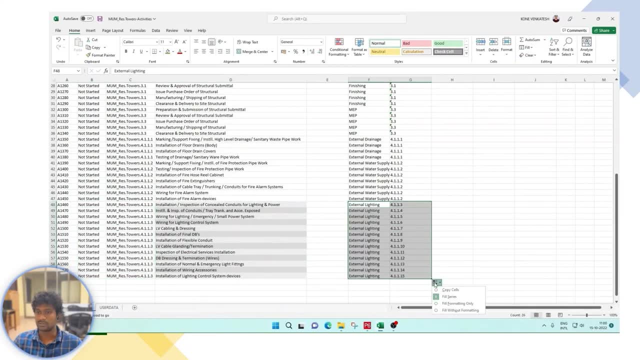 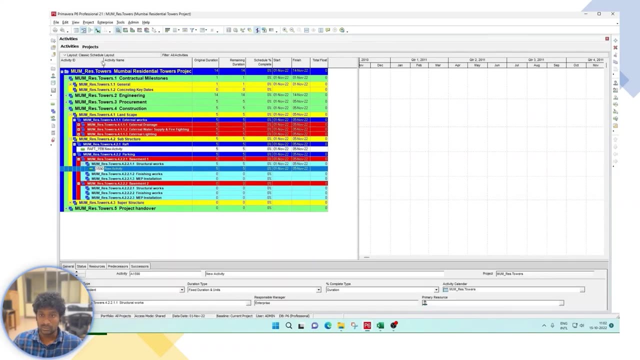 activities into the software, with the activity id and activity name and also activity duration. again, this duration, it depends upon the number of resources assigned to you, assigned to your particular activity. you may find some one that one activity can be applied in a particular way. so, for example, if you want to complete a project, you can take four days using the four workers. 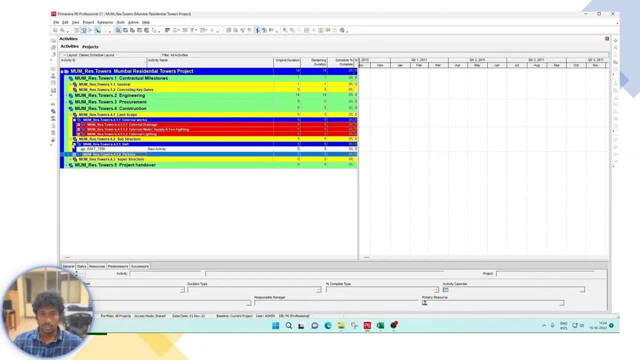 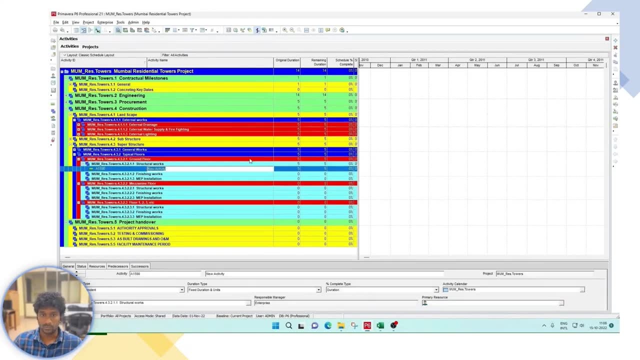 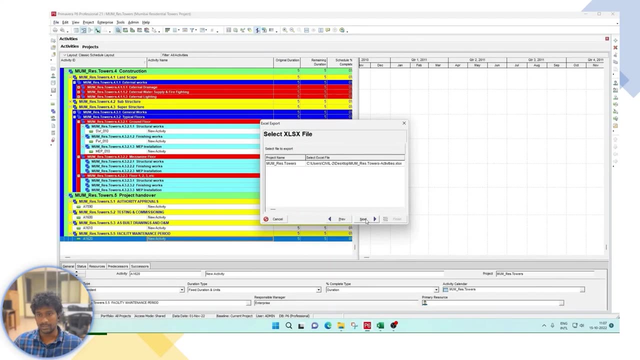 and the same activity can complete in two days. when you assign the eight workers to finish the complete project, we need at least hundreds to sometimes thousands activities into your project. so there are ways to simplify this process by we can use the excel sheet by adding the activities in the primary basic software. so in out of thousands activity, the 90%. 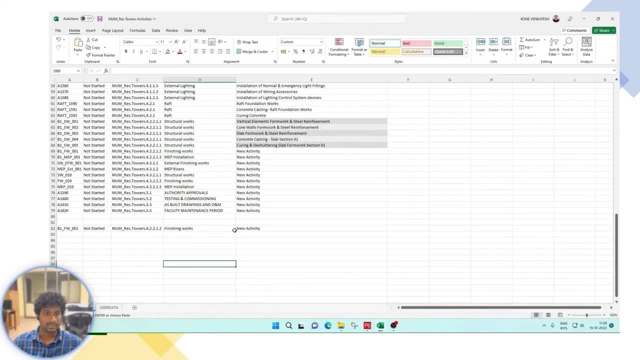 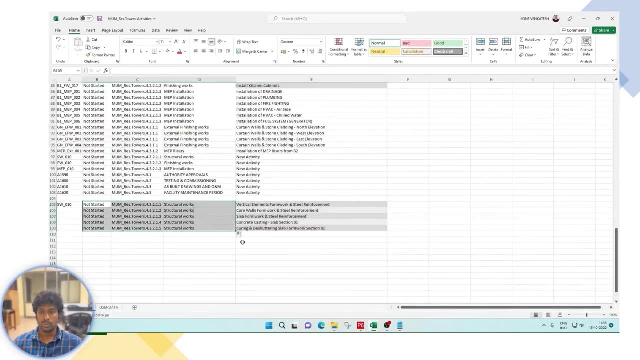 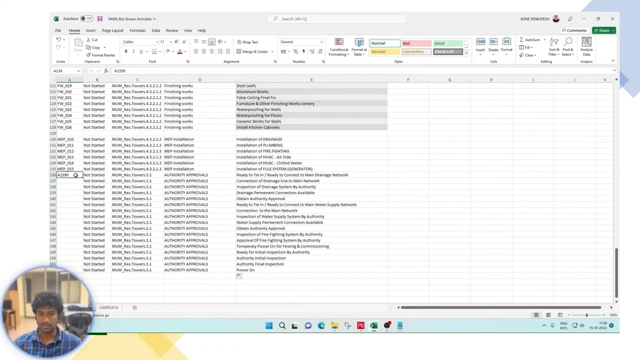 of factors are repeated. the activity that are used in the first floor was the same for the remaining force, so maybe the start date and end date will change. primary. given feasibility to copy and paste these repetitive tasks, there are some tips to follow while adding all these activities. okay, so we must. 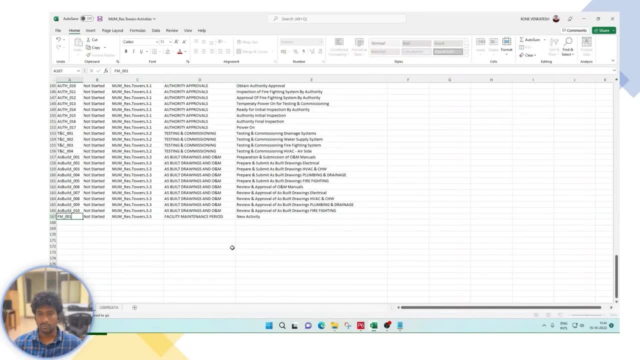 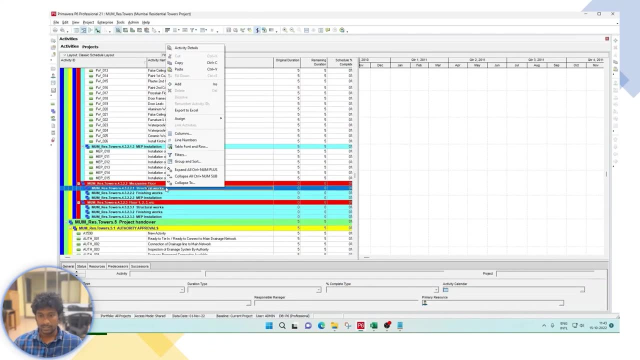 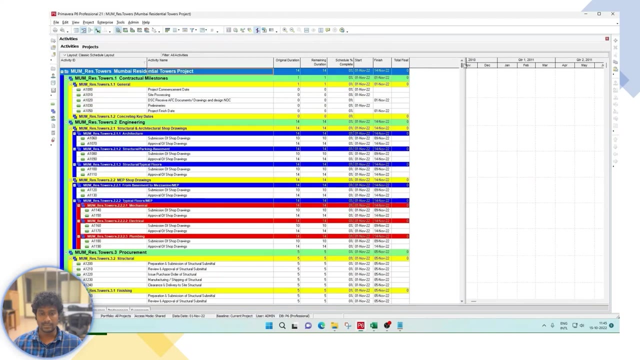 have a clear cut knowledge on each and every activity before entering into the project. so once you're done all adding all the activities, you must have a clear cut knowledge on each and every activity. so that's the first step, and then the second step is connecting all the activities with the logic links. 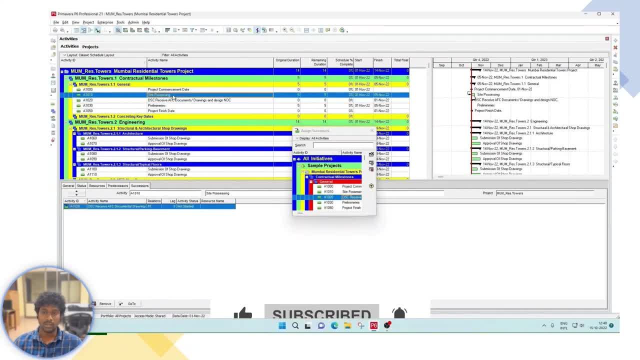 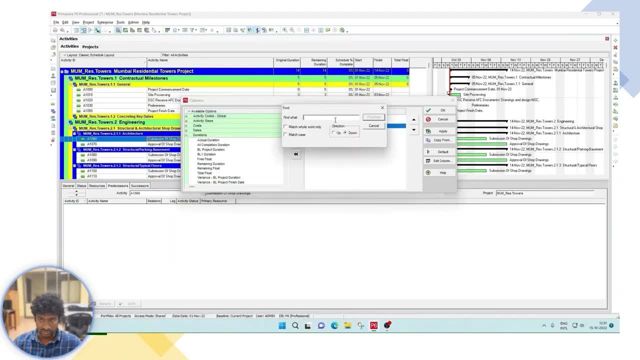 that is the step number five, or giving a relationship between the activities. there are four kind of relations. you can assign two different activities like finish to start. that means one activity is finished immediately. next activity will start. finish to finish, start to start and start to finish. this is the place you must have a proper knowledge on activities. so the 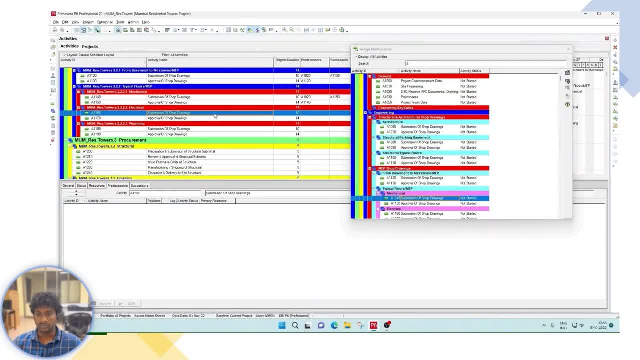 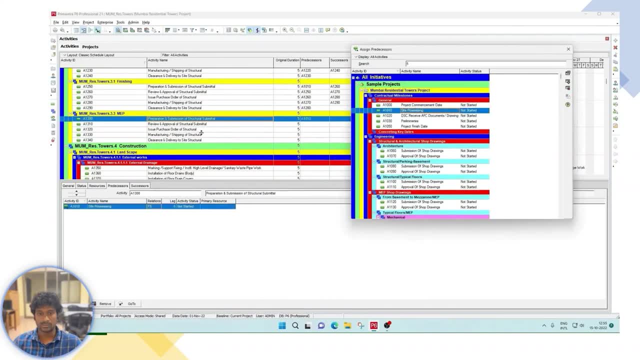 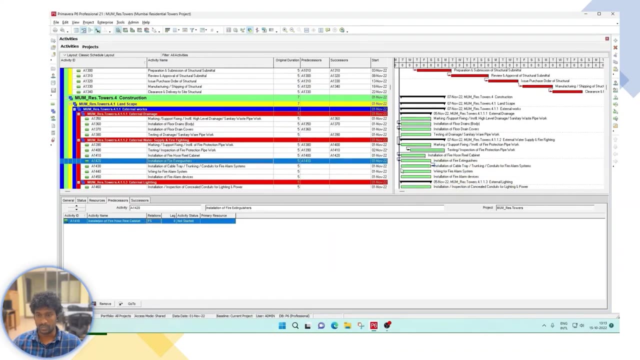 relationship is very important. so that's the first step. the third step is the first step and the third one the last step, and this is very important to define your sequence of uh and also the project duration also. once done you will. once done this uh, you will have a network diagram connecting all the activities. 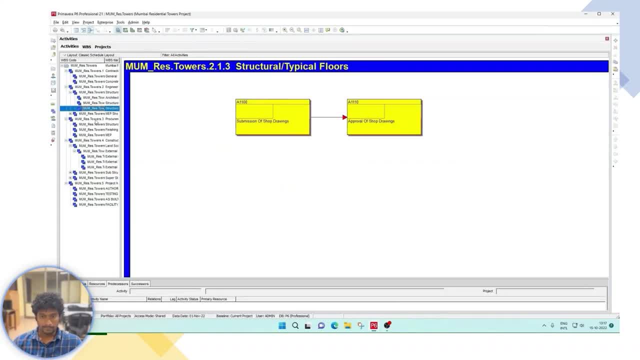 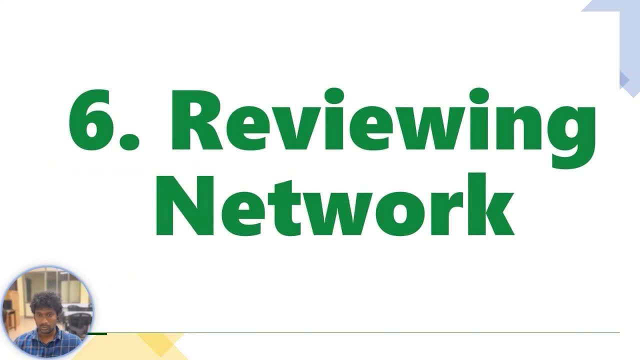 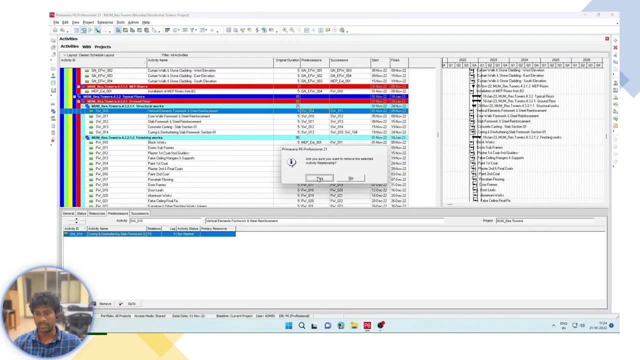 in your project. again, there are multiple ways to connect each and every activity. once you don't all these connection, okay. the next job is we need to review the network diagram, connected with one another or not. otherwise it is very difficult to find the start and end data of 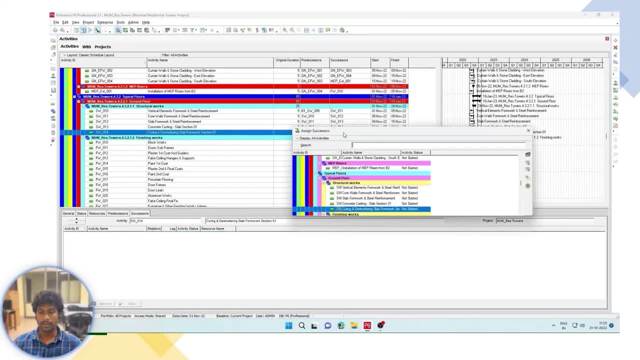 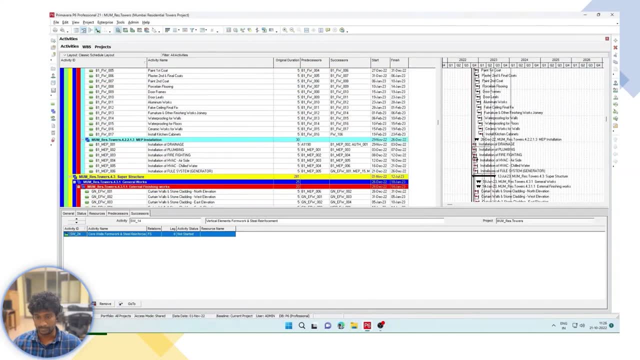 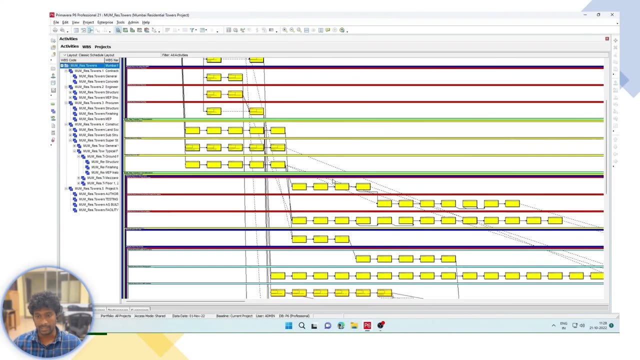 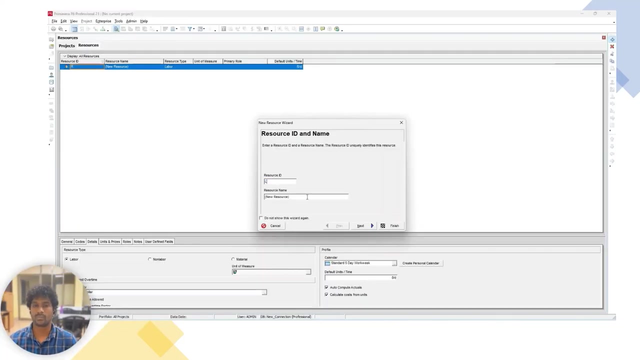 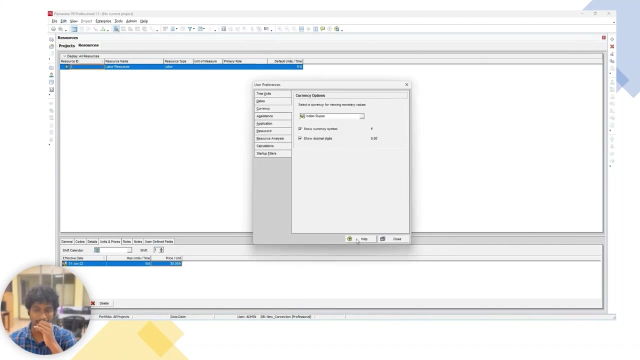 activities and also it is very difficult to calculate the critical path which decides the total project duration. by using a special features, we can review every activities, every activity, in a network diagram. step number seven is creating a resources. resources are something or some material or some equipment or some people that is required to complete the activity. 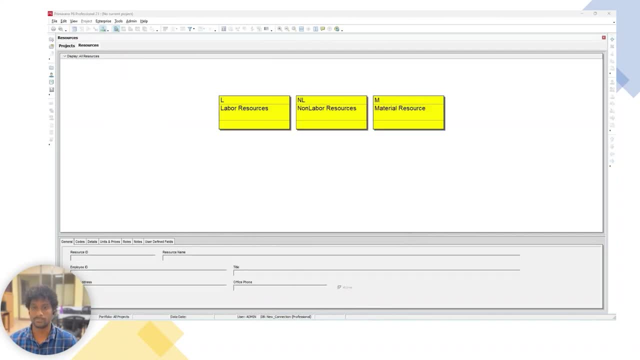 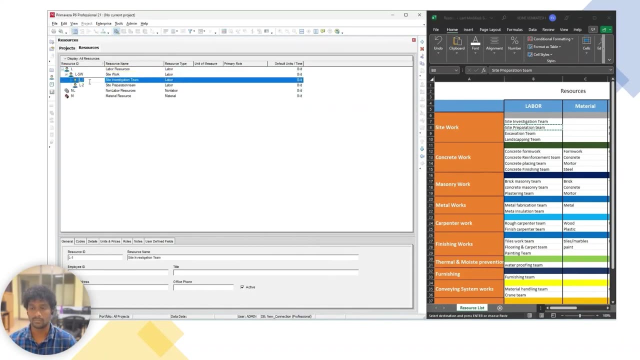 it is one of the the most important step in a project scheduling. creating a resources means to identify all the resources with the details, like a unit of measure, whether the cubic meter, the square meter, or other information that is required to complete the activity meter, or returns or numbers. so price per unit and the nature of resources. this information. 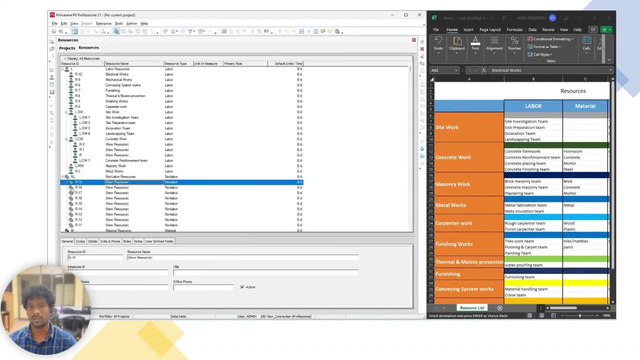 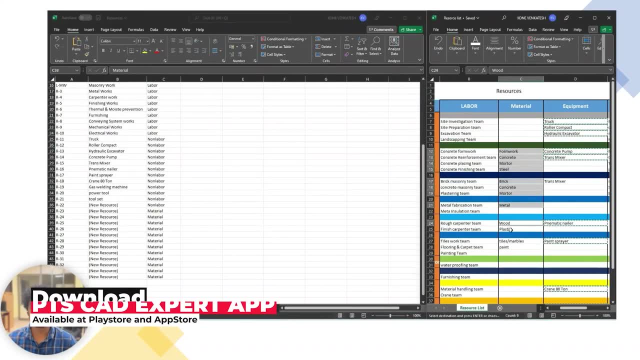 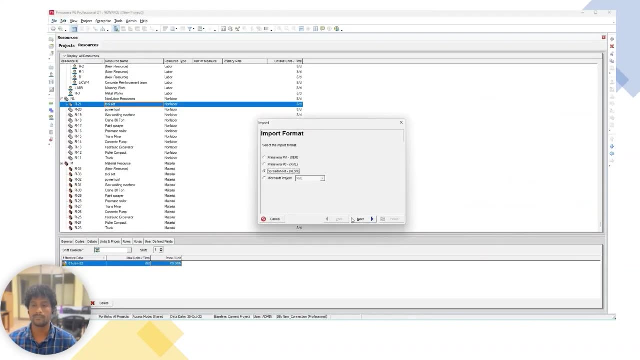 is to be loaded in each against each resources. entering the cost rate for each resource enables you to conduct a resource cost analysis. this is also important information when you are planning to estimate your project in accurate estimation. if you want accurate estimate, this resource cost information is very much is needed because you know the major portion of your project budget is. 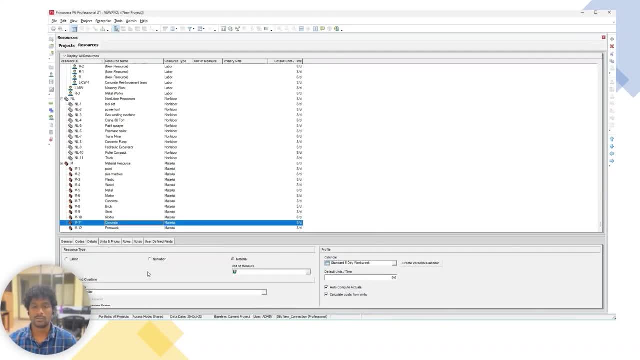 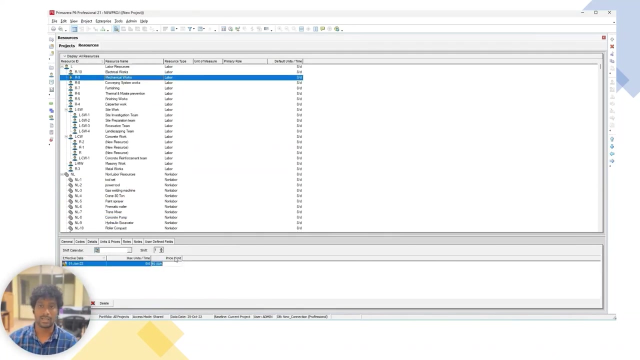 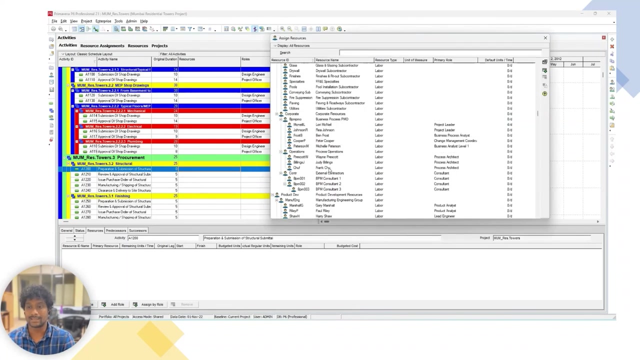 close to the resource cost only. so some resources are very limited in availability, like labor resources. so once you create all resources- the manpower and materials and equipment- next job is to assign these resources to the the relevant activities. that is the step number eight, assigning resources to the activities. the required quantity of each resource is assigned to. 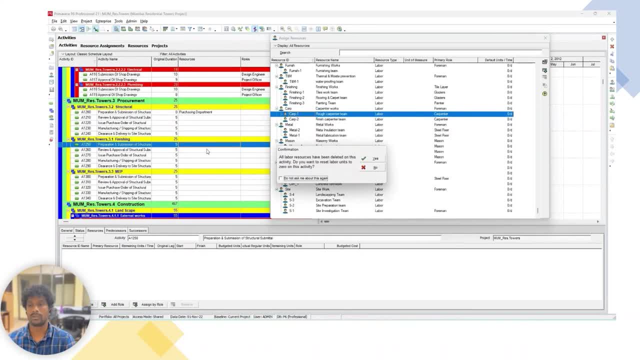 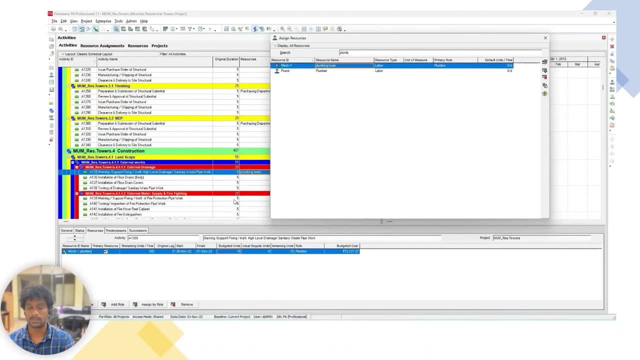 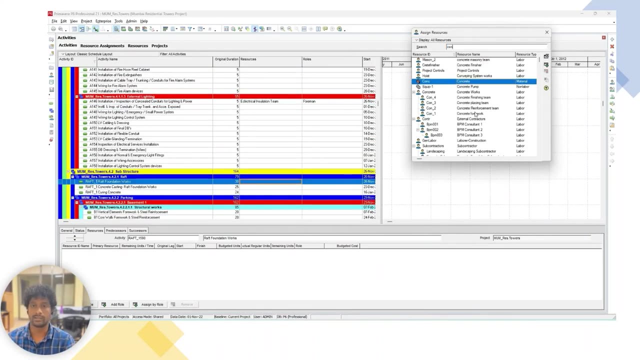 a particular activity. if suppose, uh, if you are placing some concrete, okay, 30 cubic meter of concrete is required. six peoples are required. okay, some reinforcement, some steels, some, some tons of steel is required. like that, you need to assign the required quantity against each activity. for a slab, a column, how much concrete, how much, how many. 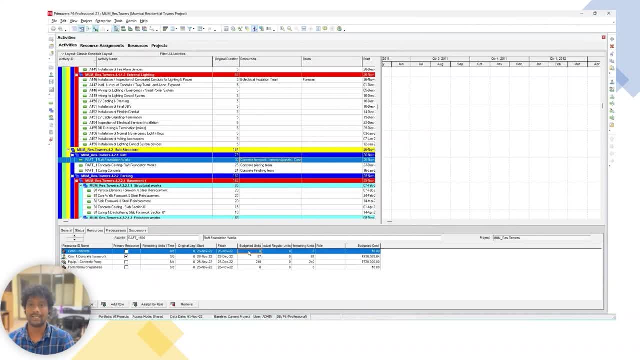 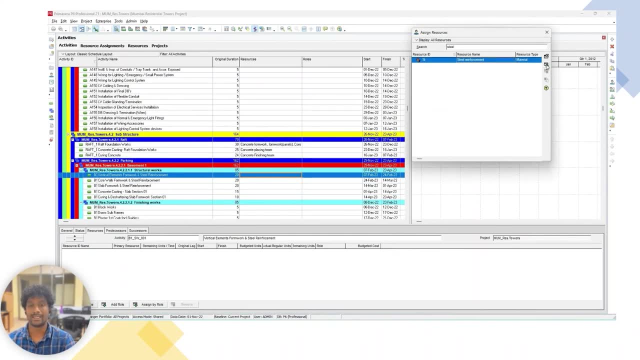 levels. what equipment is needed? some activity may take a single resources, some activities takes more number of resources. again, it's our job to identify, uh with our site experience. again, there are tricks and there are tricks to simplify these stocks by using the actual shader and after assigning the resources, we need to create and use the roles. step number nine: 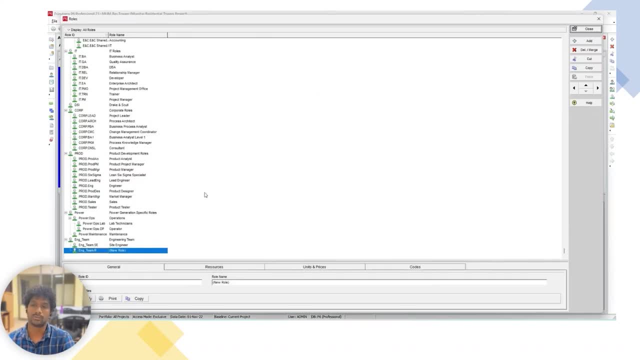 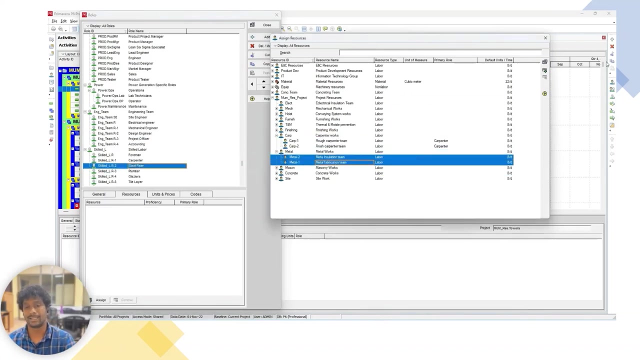 primary as an additional function, the orbital cost, the roles which is used for planning and managing the resources related to the people, like top management peoples managing the employees in the organization, like site engineer, design engineers, accountant or draft man, something like that. so the role, that means the role maybe the skill or a trade or your job description. the role may be. 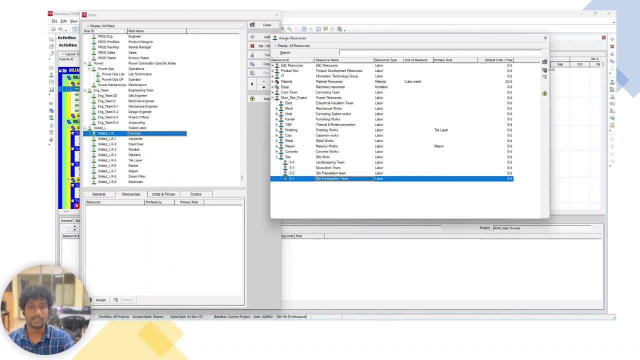 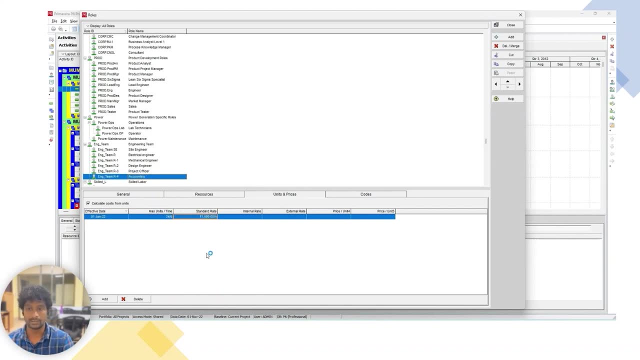 assigned to activities in way similar mh, how they work and at the time of application, FPS pattern or by the way the resources are assigned. some activities like inspection- inspection of plumbing and something- approval of drawings- so these are activities is done by the skilled peoples and the roles the 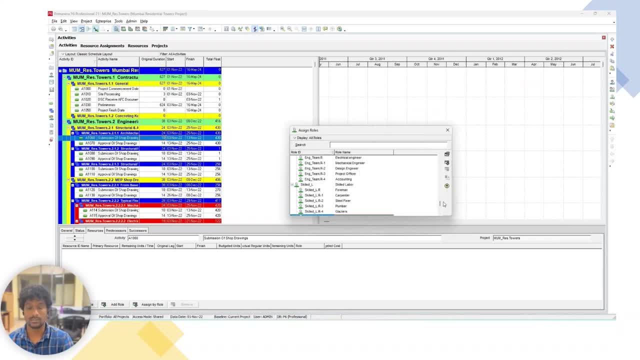 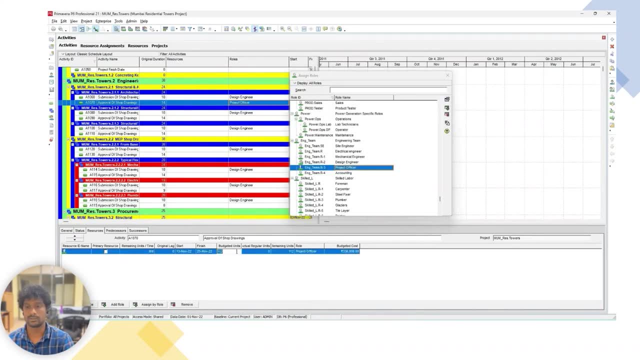 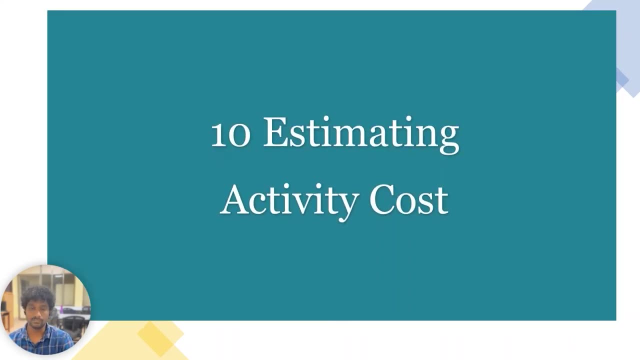 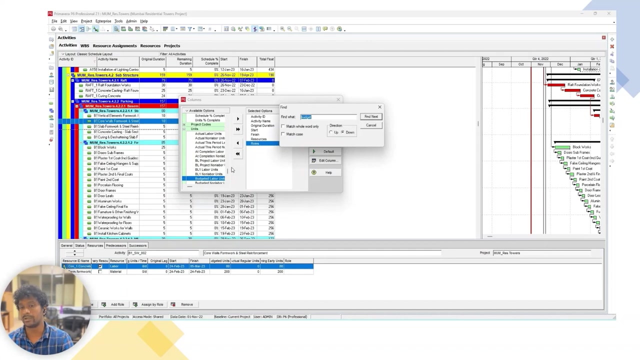 roles can be used here in the resources in the unit as an activities to these roles. once you've done activity resources and activities roles, the next job is estimating the activity cost. once you assign the resources and roles to the activity with the cost information and then primary help, you get the cost of each activity. that information you can visualize in. 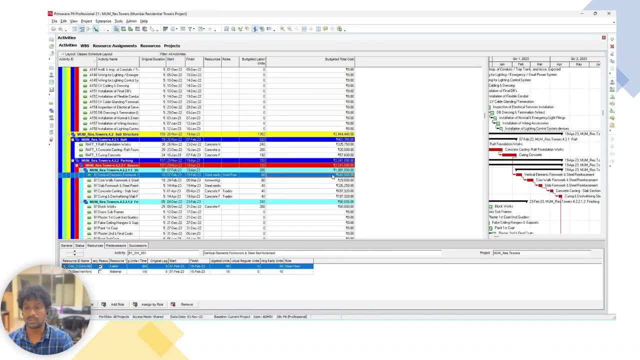 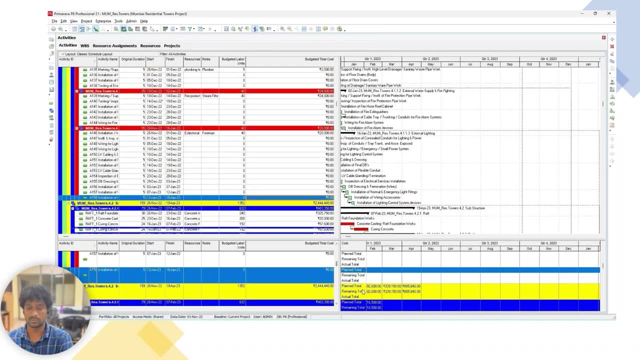 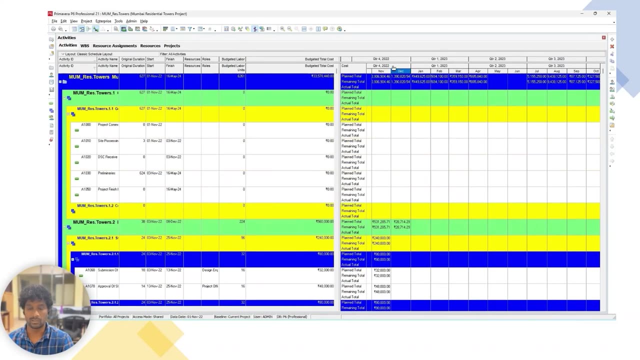 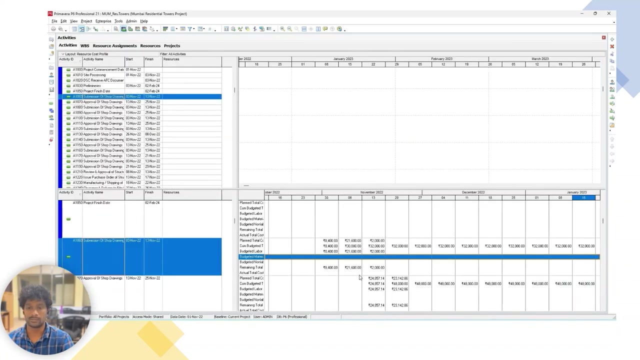 the form of tables or in a crop, against each activity. for a particular activity, how much it is cost. okay, what is the labor cost? what is the activity cost? equipment cost, what is the materials cost? like that you can display every information in a primary software and there is a column you can add a direct cost in the name of expenses. but with some. 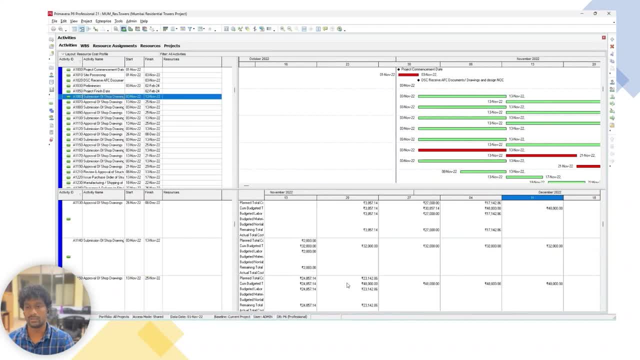 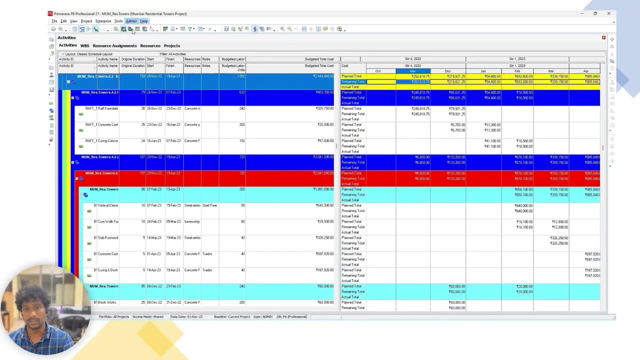 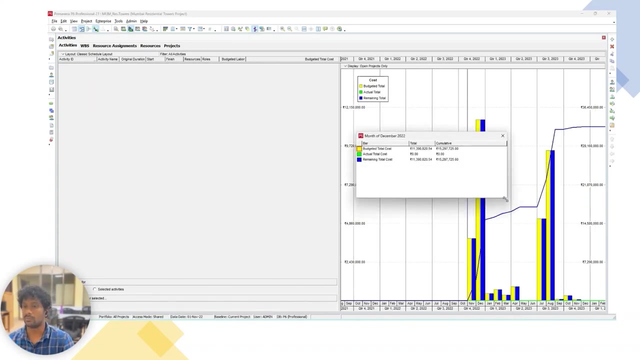 costs. it is very difficult to identify the resources. you can directly. some indirect cost will be there. okay, so that you can examine the 11 that prepared time- uh, preparing the time-based cash flows: expected cash required in a day or a week or a month during the project execution. 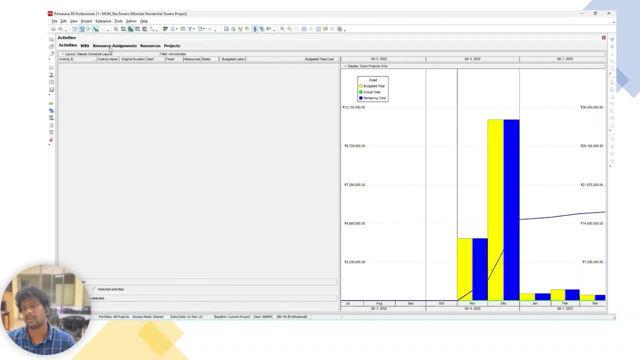 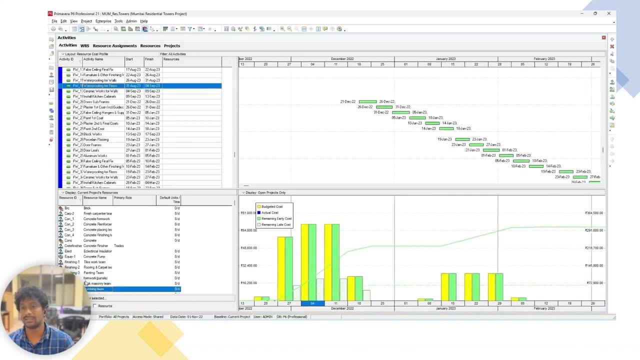 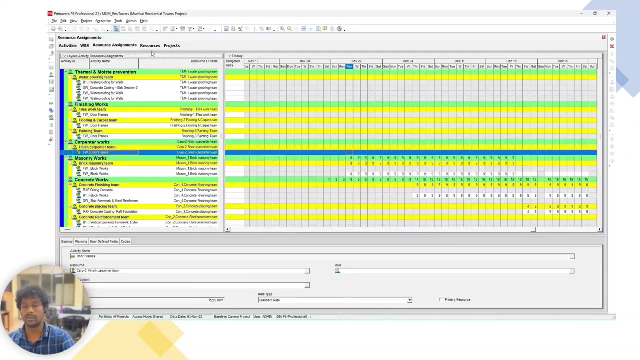 it is good to have idea before execution how much cash is required in monthly ways, or sometimes week-wise. so, based on that, organization can manage their internal and external funding options. otherwise the activities may delay. lack of funding: the developing resource usage profile. so this is a similar way of exposing the cash flows. 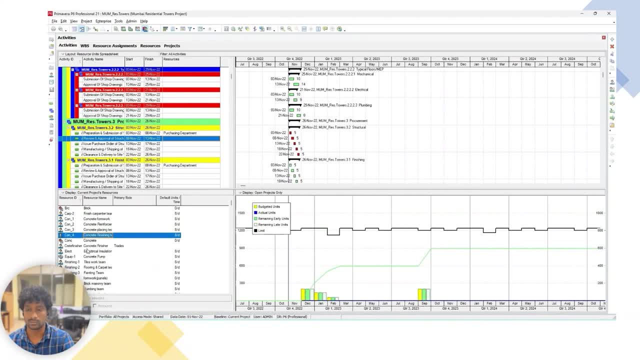 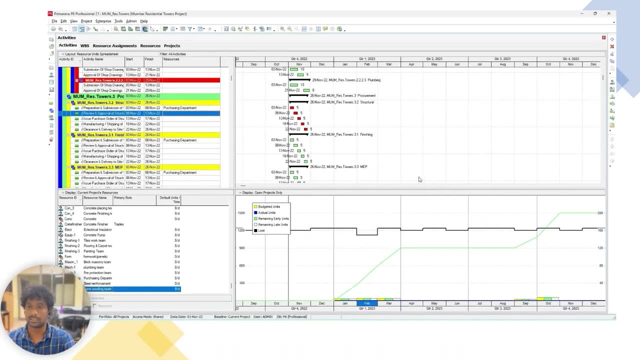 there are several ways of motivating the cash flow over this activity. like that, the cash flow rate may be high, so that the cash flow rates are more likely in maximum period when you collect the cash flow rate. how much cash should be spent to remove the cash flow rate? 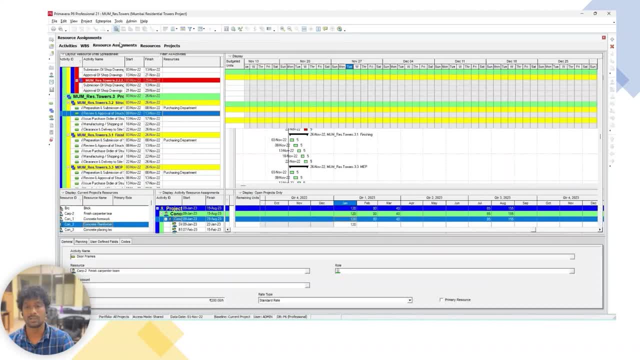 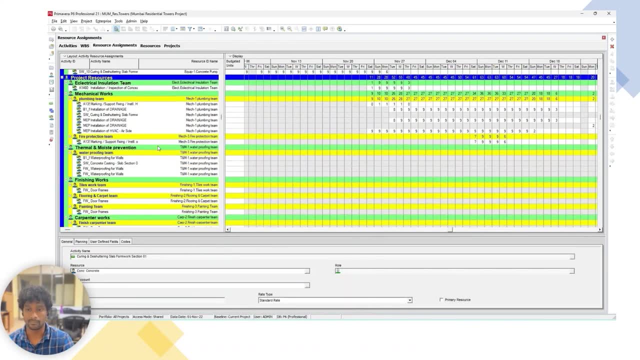 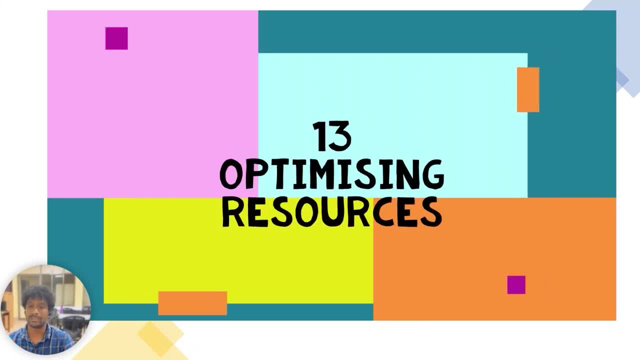 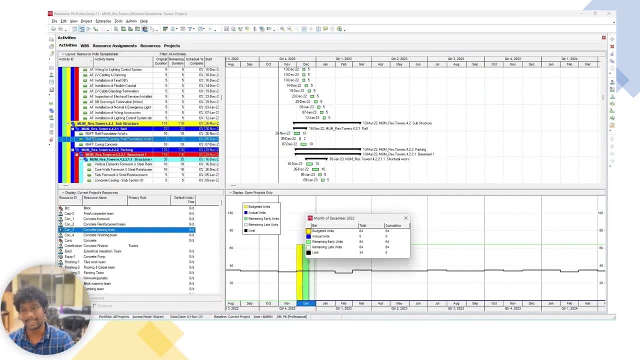 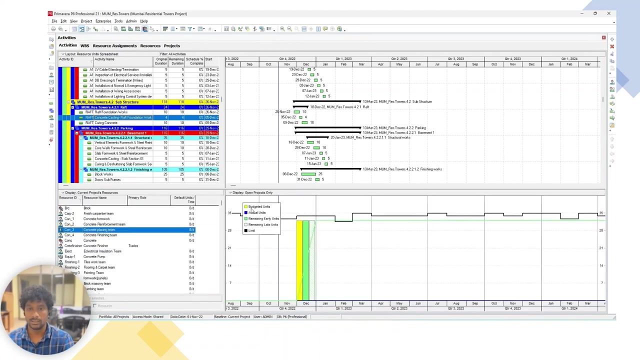 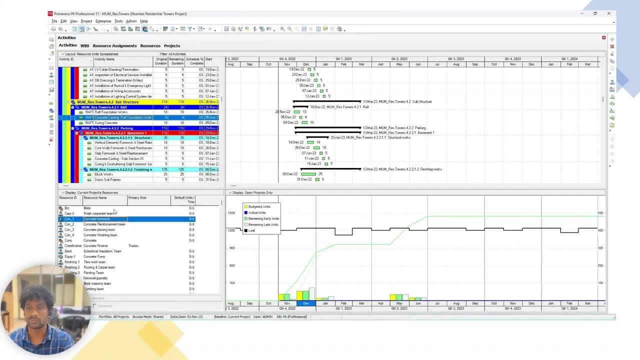 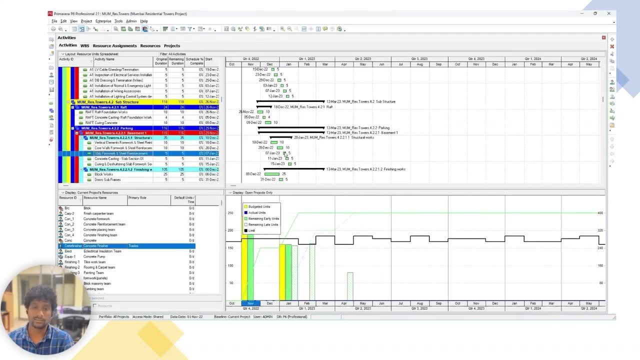 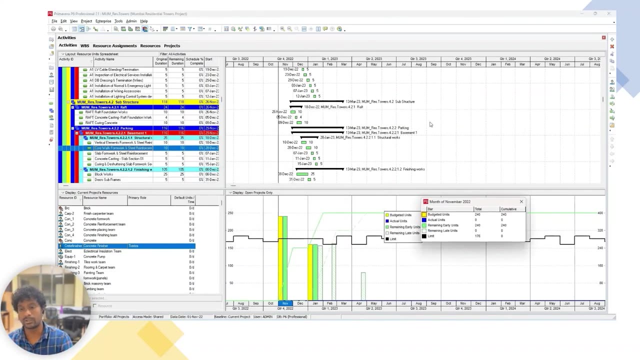 the function is simple, like delaying the activities until resource becomes available. this is the thing that you need to do in the resource leveling in some cases. another techniques we can use, like resource smoothing. so here time is fixed. the project duration is fixed, so here we need to add a lot. we need to allow extra resource to complete the activity on time. 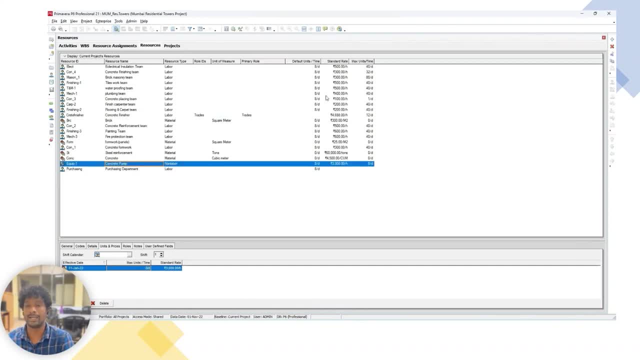 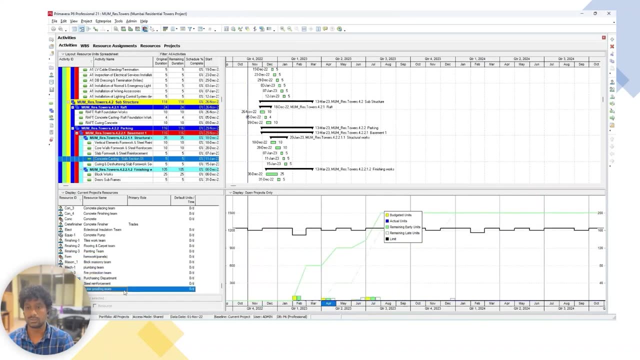 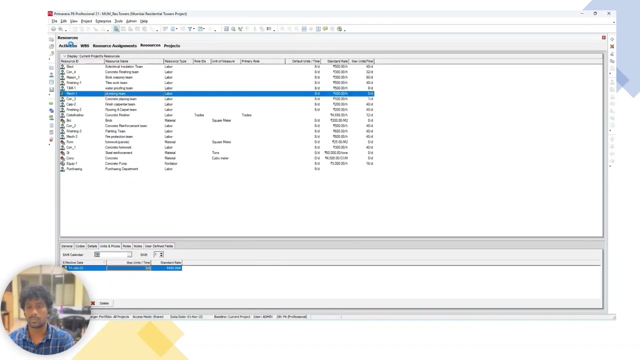 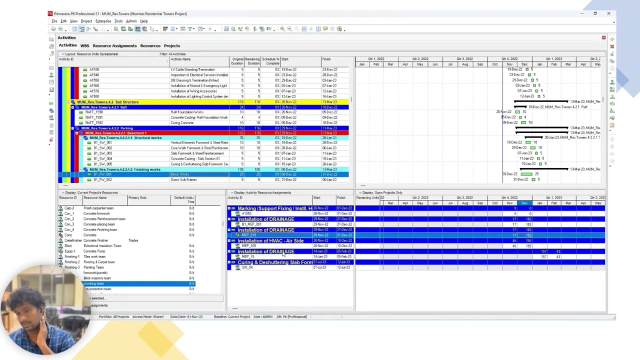 if suppose one activity is there, it required eight days by using the four workers. so but we can. i want to reduce the project duration so i can, i can give extra resource, like eight people, so i can complete that particular activity in four days. so where the projects are important, the date time is a constraint that this technique is. 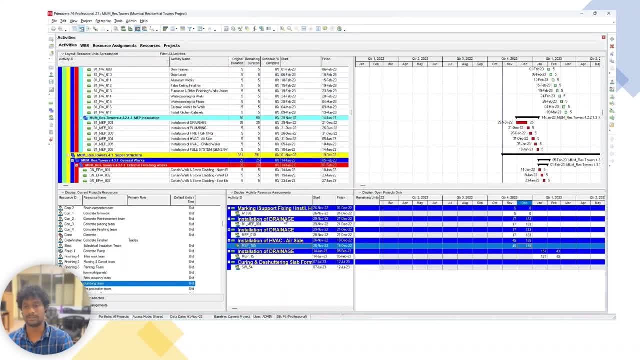 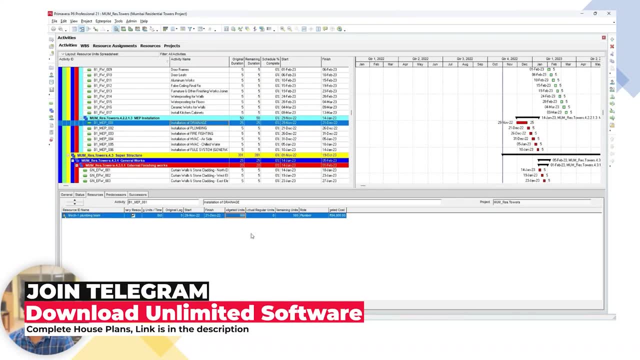 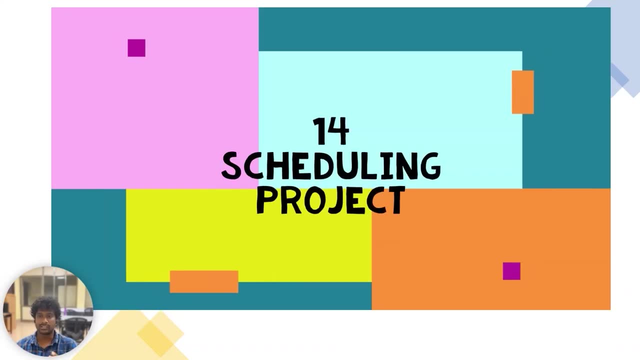 used resource level. you don't need to worry about all this concept. i dedicate one module for this purpose. as an input module, i will teach you all the concepts failed in this module. in this step, the software calculates the short test time in which the project may be. 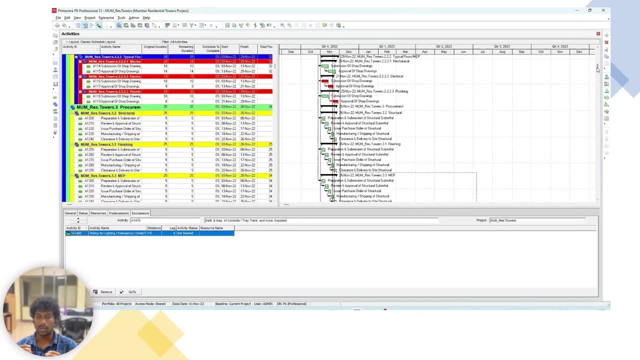 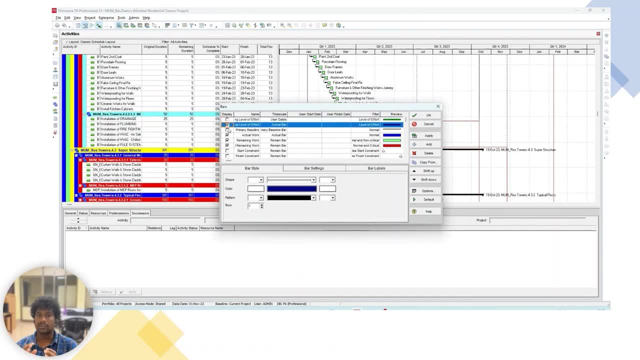 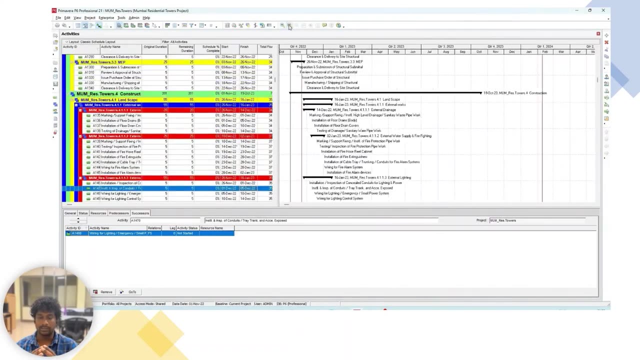 completed and also it will identify the critical path by connecting the critical activities which are represented in red colored bars. this is the third phase in a project scheduling. in the first phase, till the step number six, to add at the activities and and connected with the logic and the second phase, you added the resources and optimized it. so in the second phase, you added the resources and optimized it. 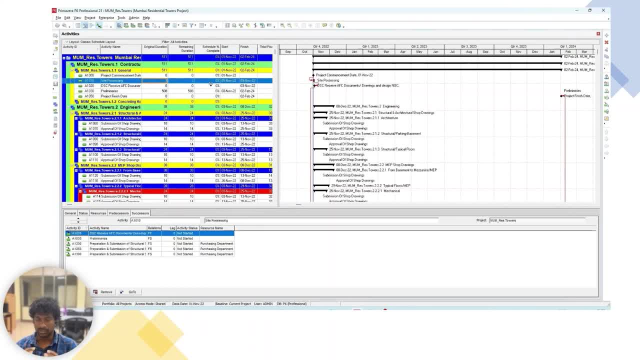 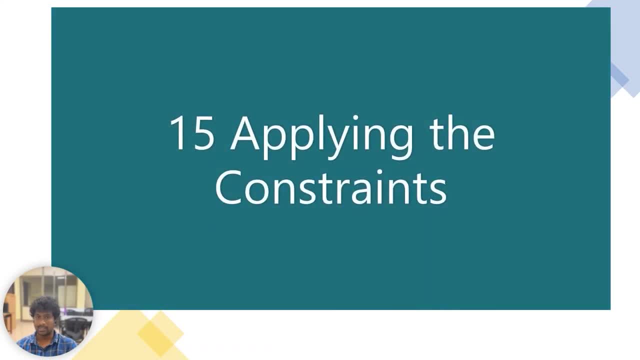 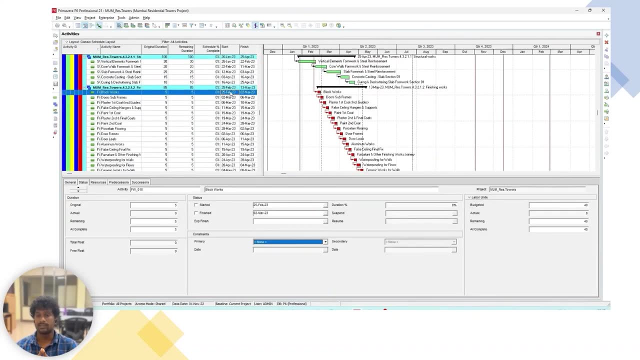 by using the f9 shortcut for scheduling, third phase will start and the next step is applying the constraints in the project. constraints means the date that restrict the start are complete of an activity. there are two types of constraints: or external constraints or internal constraints. external constraints are the contractual dates. 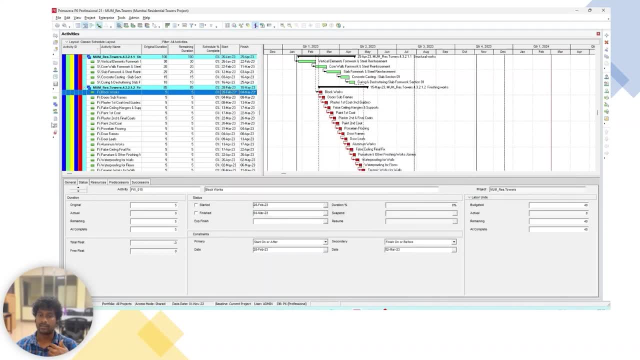 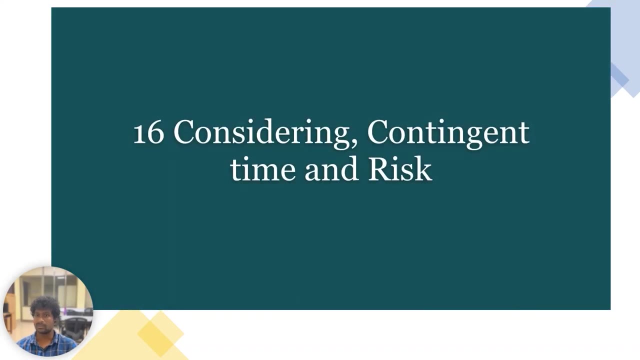 you must finish the work package in a particular day. internals, like resource constraints, and you need to plan the activity by constraints, by considering all these constraints, and the next step is a optional step that is, considering the contingent time and the risk. so this is optional steps in a project scheduling. 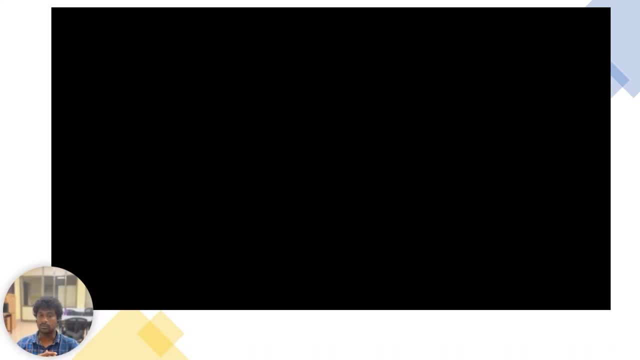 the process of planning in a project. in the process of planning a project, you may identify the different risk. so so we need to perform the formal risk analysis. so in this formal as risk analysis, you may identify the mitigation activities that should be added to the project scheduling. before, before the approval, the addition contingent time should be considered. 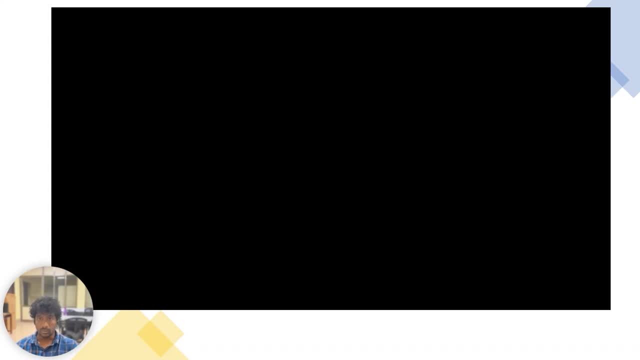 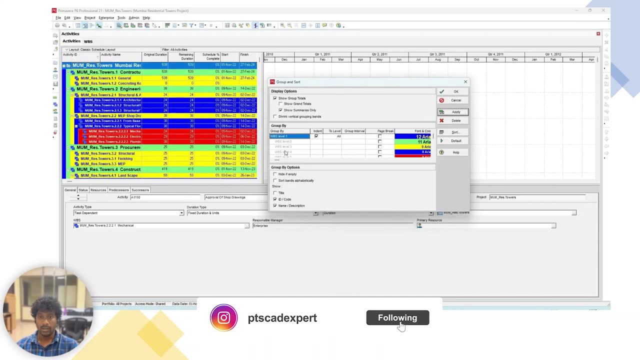 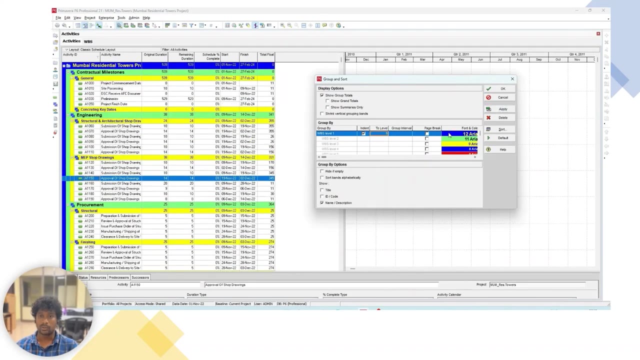 when submitting a schedule for a approval. so this, this complete step, is optional. so next step is organizing the project data. it is it is important to display the project data. what we exactly needed to analyze the project data may be the activities with the start and finish dates or activity. 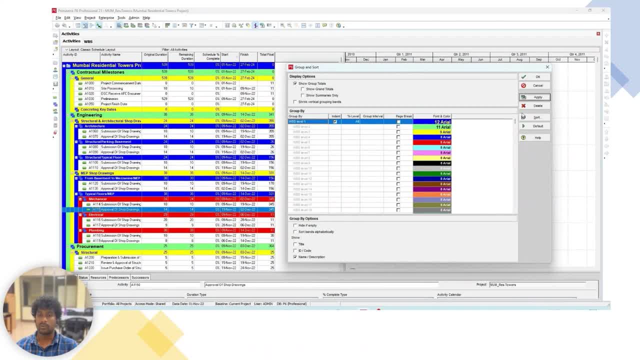 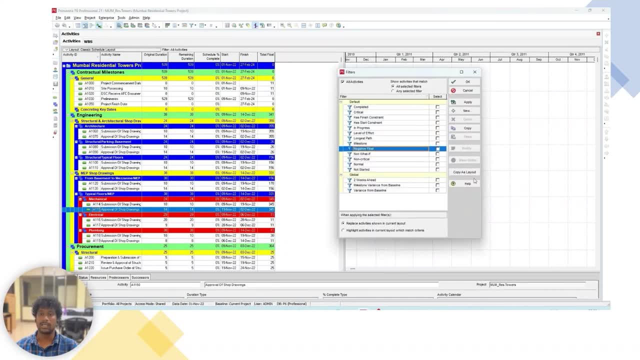 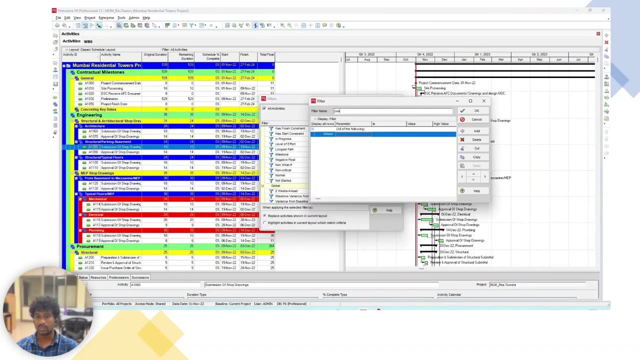 with the plan cost or a cash flows. so with the help of features like a group and filtering and shorting options and, more importantly, using the layouts, we can customize the display as like we want. and the next step is the printing and publishing these data. once you organize the 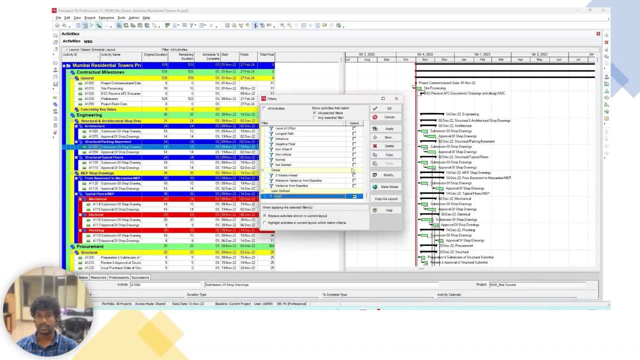 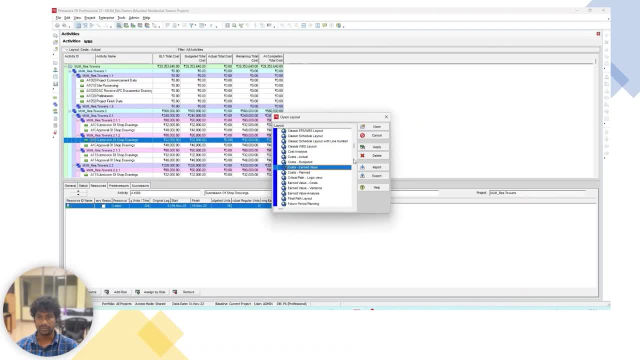 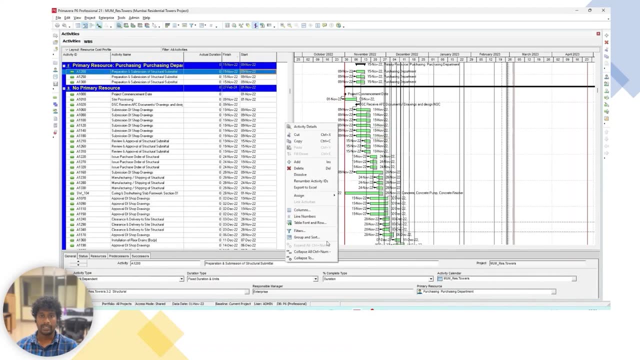 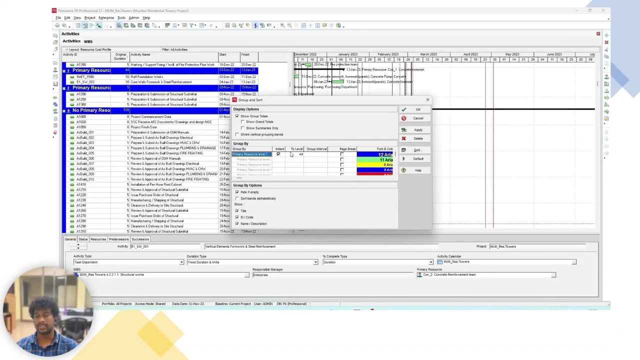 your project data, so how you want to look at. then you need to print the data and publish the data into different in the different platforms. that is step number 18: printing and publishing. this step is for to communicate information with the other stakeholders before finalizing the plan. 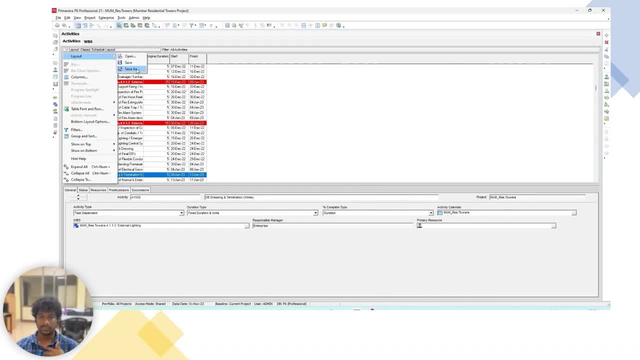 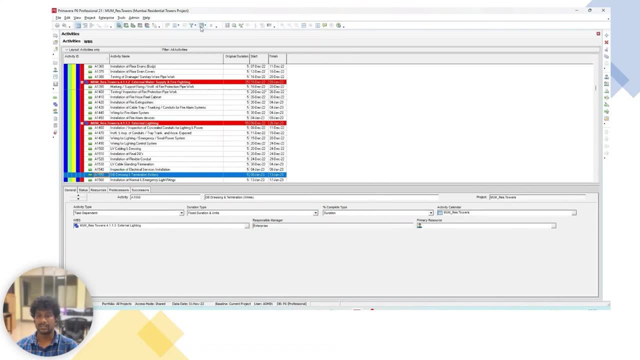 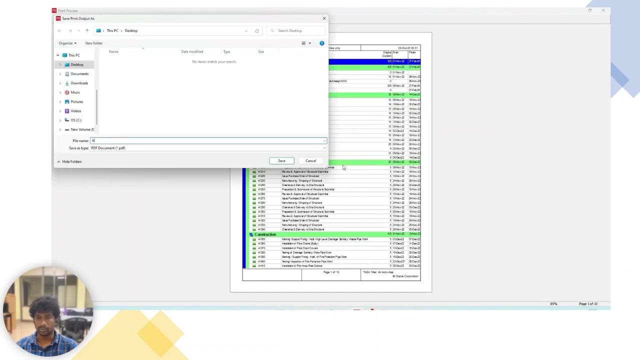 we can't share the primary files to all the peoples. instead of that, we print and publish the data that is required to check and forward to the people. this is the final step in the third phase from this planned part is completed. the next phase is monitoring and controlling the project. 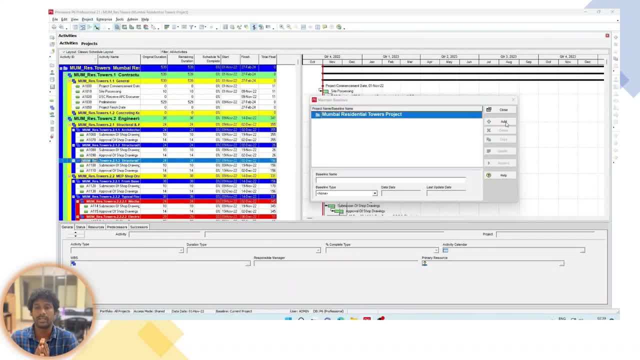 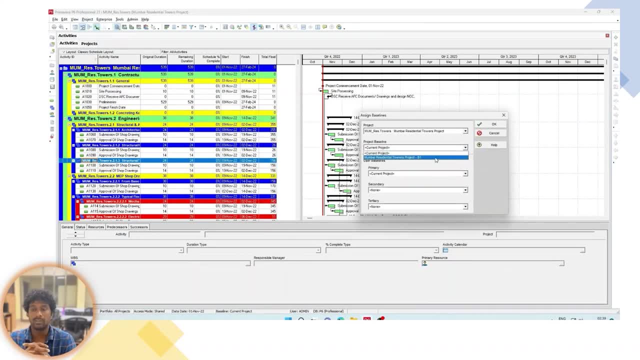 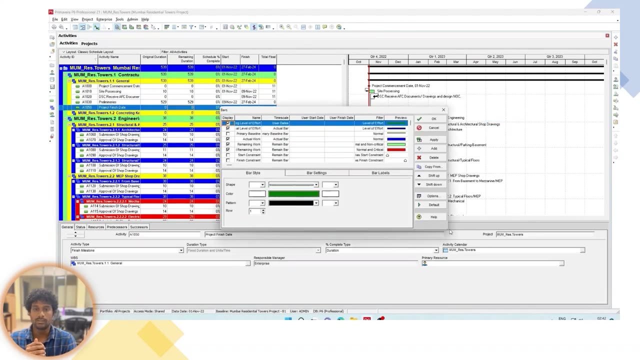 the baseline. so this is the first step in monitoring and controlling the project phase. so the optimized and agreed plan is used as a baseline for measuring the progress and the identity changes, monitoring the changes in the project, the software, the software record the baseline dates of each act. 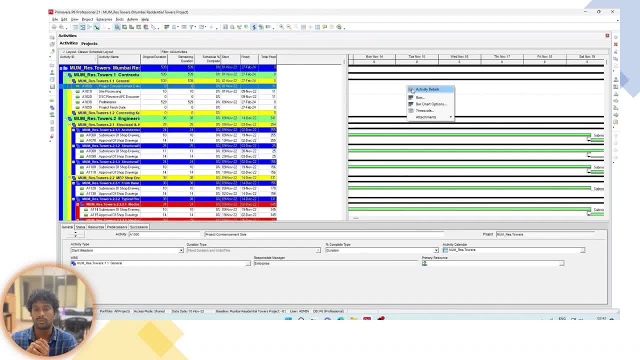 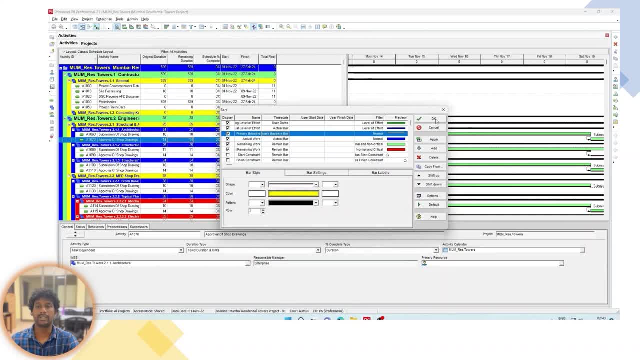 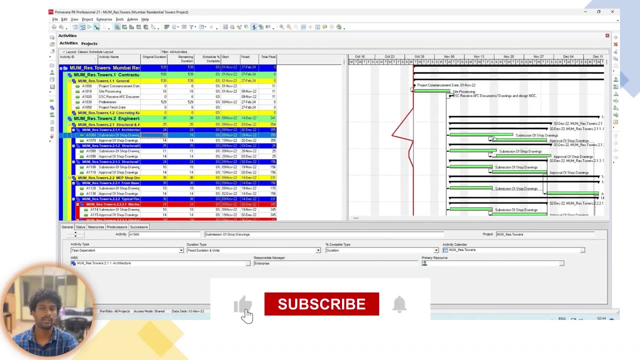 activity for comparison against the actual progress during the life of the project. So here all you need to do in the execution phase update the progress in Primavera software once you just track the project and update in the progress. So the step number 20 is updating the progress. 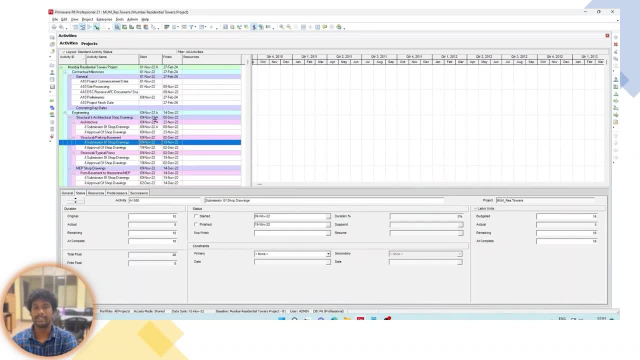 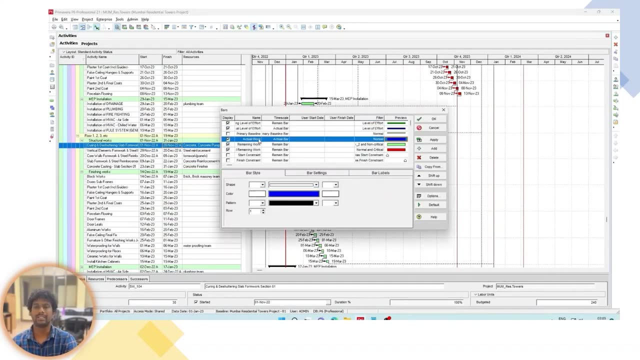 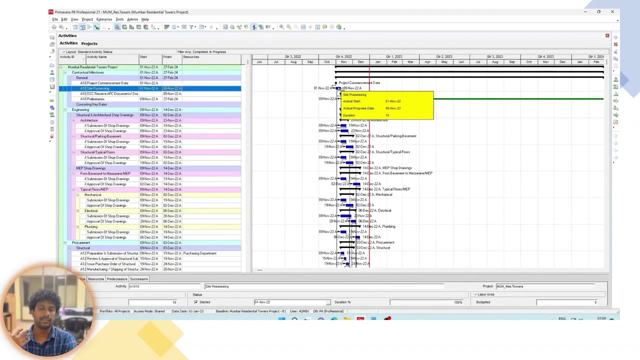 This is the important phase for the regular monitoring and control and it will begins with tracking the progress. So normally the project is updated once a week, bi-weekly or monthly and in a very short term, projects like it will complete in a days, So that those projects could be updated directly or even by shift or hour. 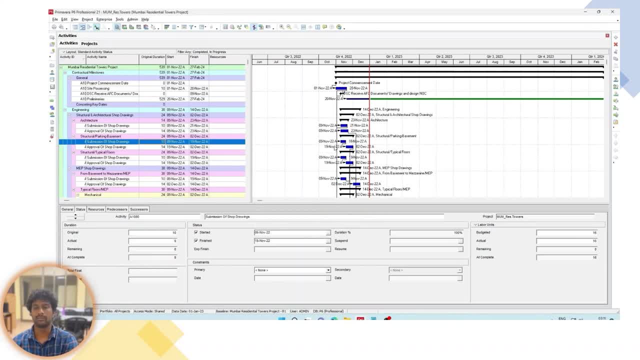 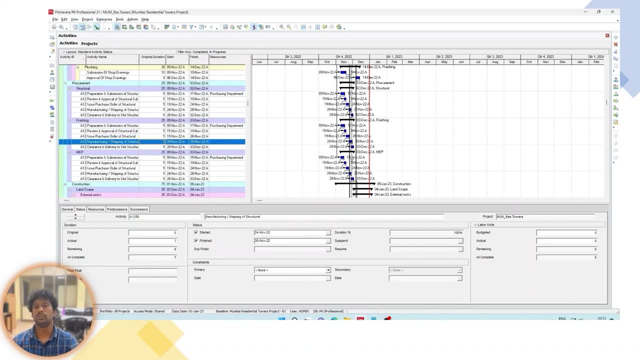 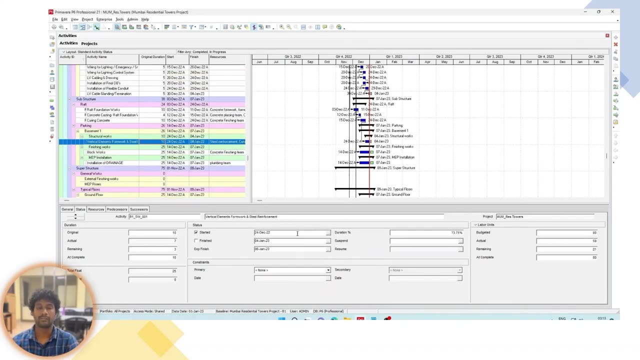 A project in a lifetime. a project can be updated, typically updated between 12 to 20 times in its lifetime. So, whatever the frequency you choose in for updating, you will have to collect some activity information in order to update the schedule. So for completed activities, so you should have an actual start and actual finish date. 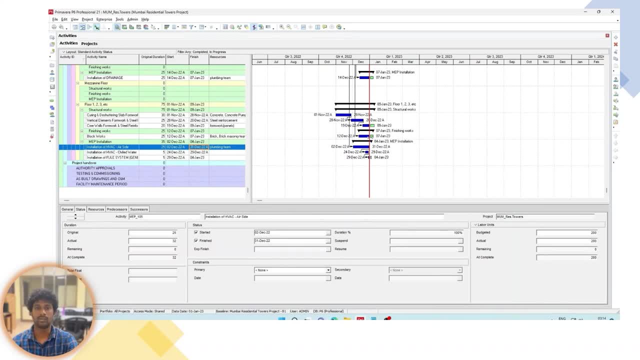 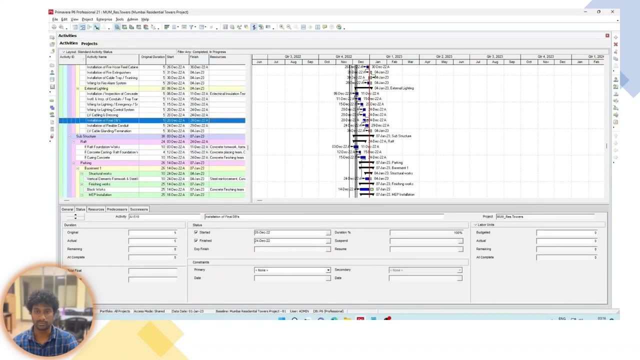 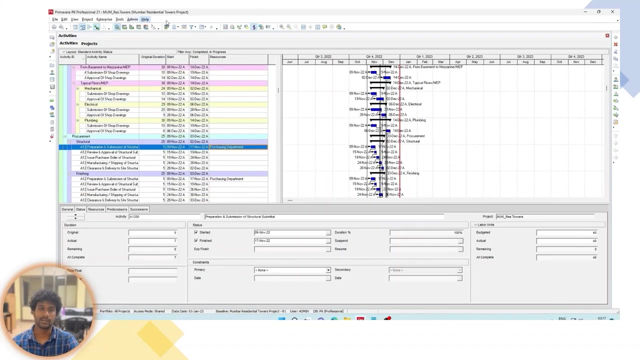 For in progress activities. you must have an actual start date of the activity, percentage of completed and expected finish date of the activity For unstarted work. so you need to check any reasons to those activities in terms of the logic and durations. Once you have done all these- updating the work, updating the progress- the next important 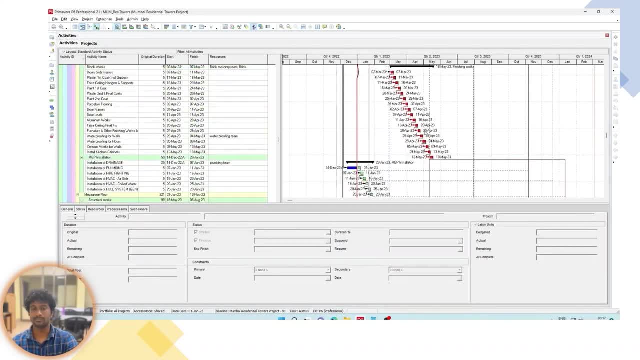 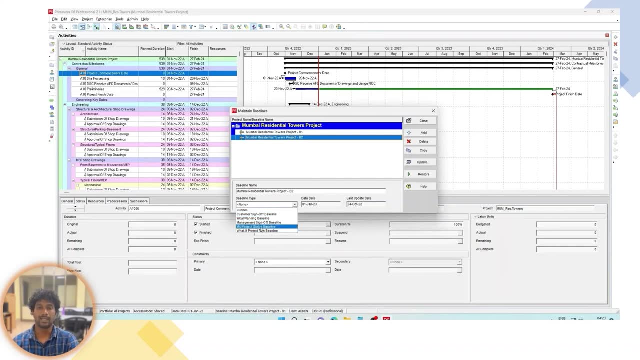 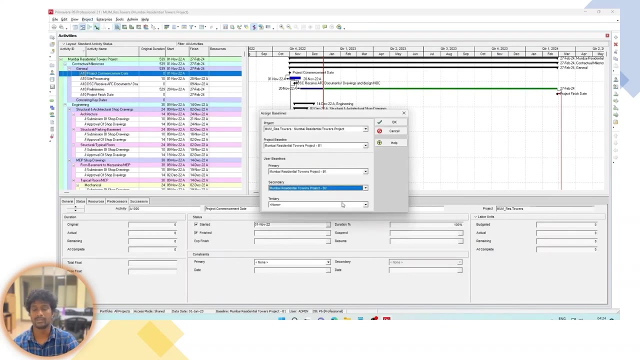 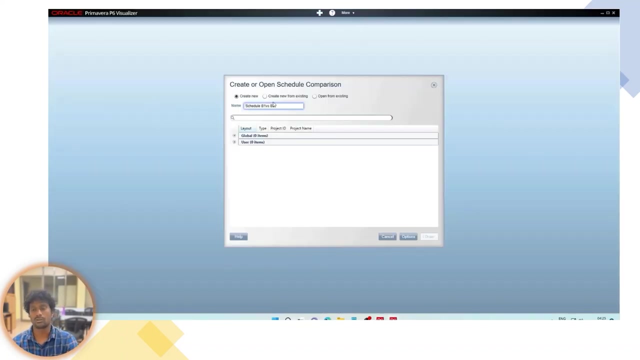 step is performing the analysis. So to understand the reality, some kind of analysis have to be performed, like comparison analysis, time comparison, the cost comparison analysis. from there you can get a schedule variance, How the schedule is vary, The plan versus an actual. likewise in the cost variance. 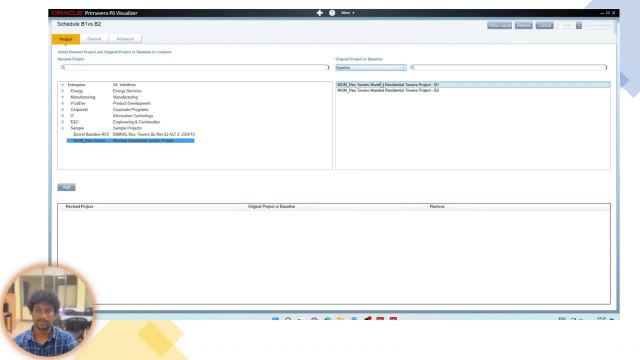 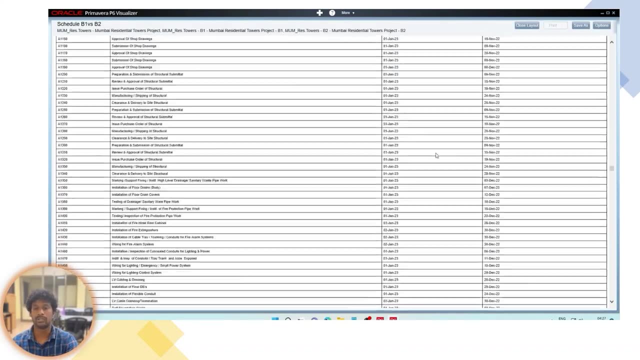 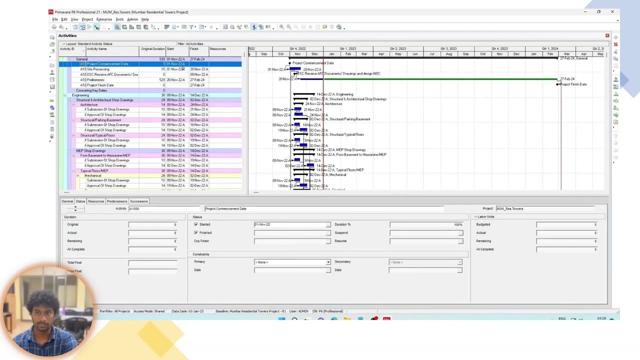 So, and also the end value analysis. this is the important analysis in the project management So for to do the end value management in the Primavera. so we need to follow the seven steps. Seven steps must be completed to set up a Primavera of basics for end value management. 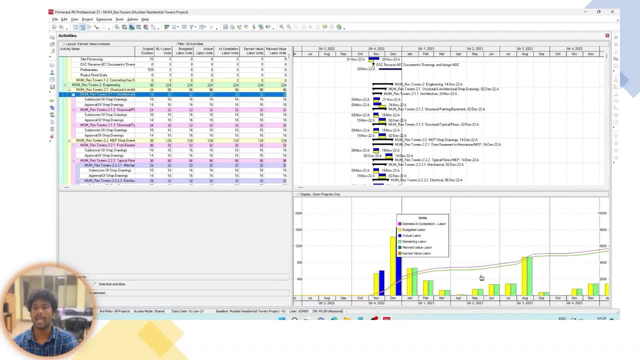 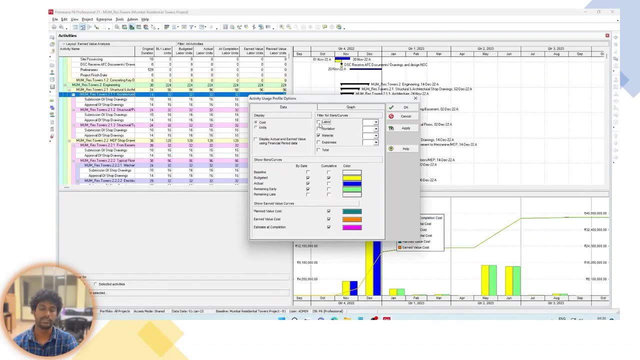 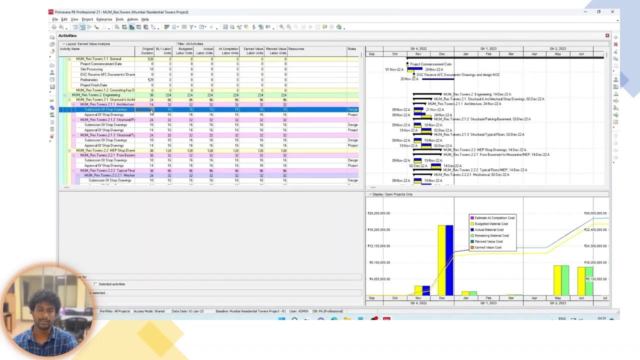 Once you done, you must have end values for all activities. End value is the monitor value that indicates the amount of work achieved on a project. If your project is 100 crores, you completed 25% of work. whether your work is finished, your work is valued 25 crores or not. 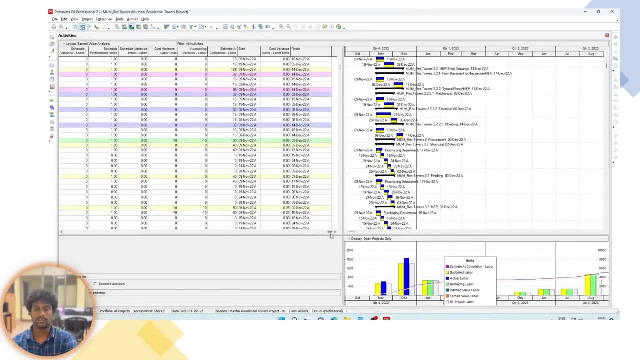 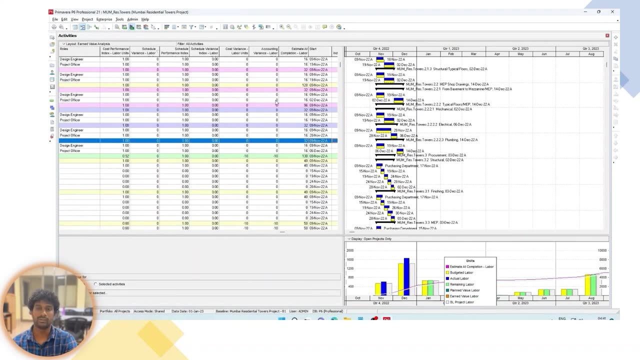 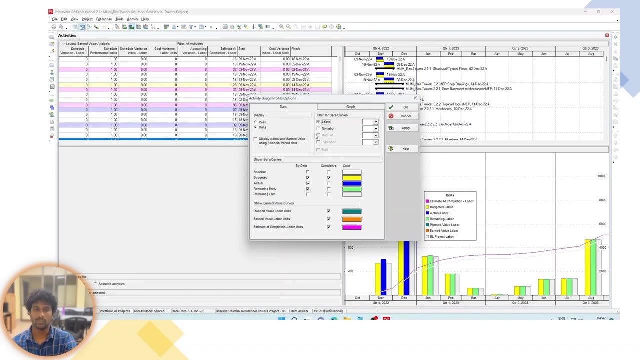 So that is the end value. So once you done all these things, okay, you identify all the changes. So you don't have performance analysis and everything. You identify some serious changes, Okay. So the next step is to identify the existing progress issues in your project scheduling. 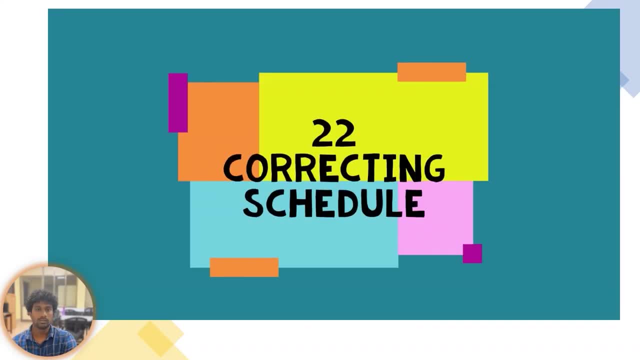 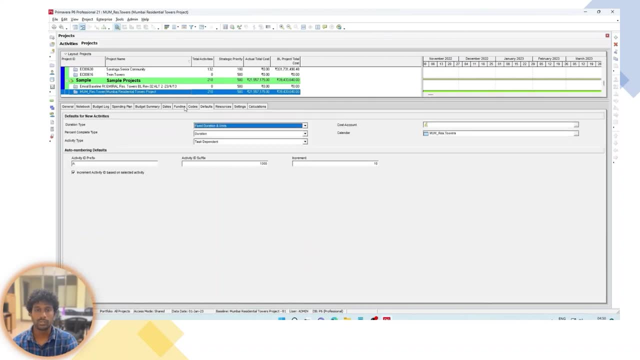 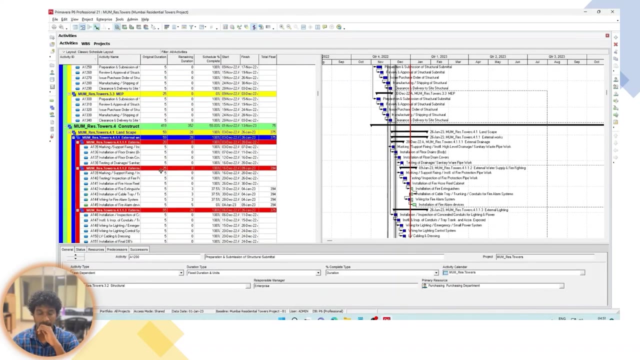 And the next step is correcting the schedule. That is step number 22.. So this can be done based on the reality. So you need to do some modification and corrective actions to control the project progress. So there are a lot of variance, a lot of changes. there is there a lot of deviation from as 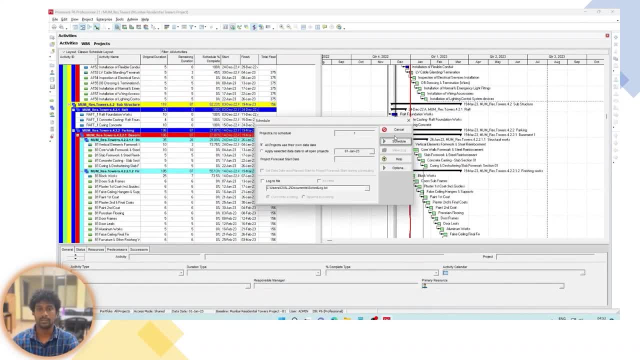 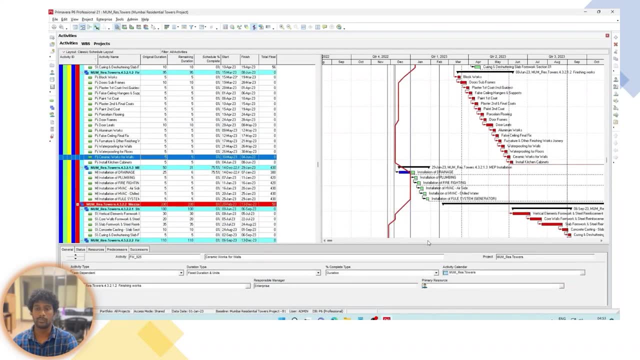 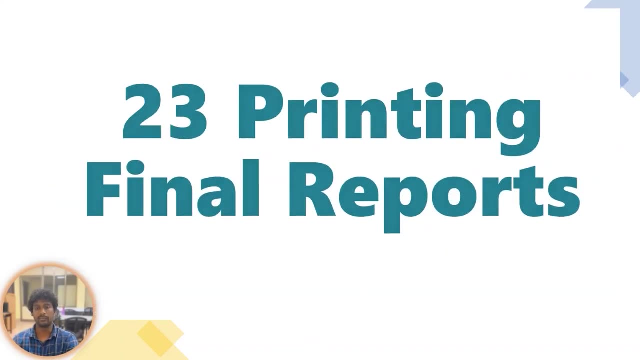 planned and actual. So for that You need to have, or you may need to make, changes in existing activities as well, as whatever is changed at this stage is to be done by approving all the important affected stakeholders. So then, what is the printing final reports? 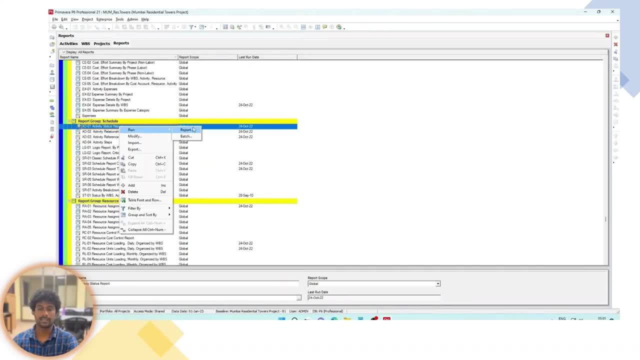 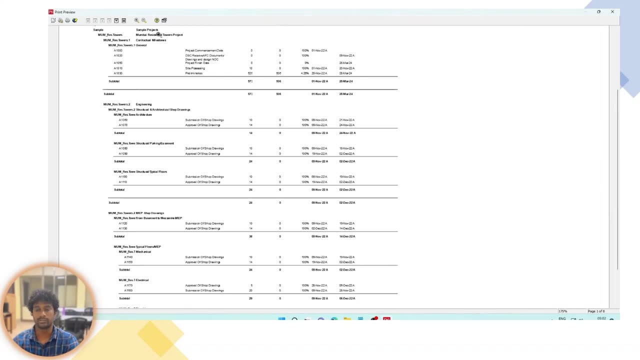 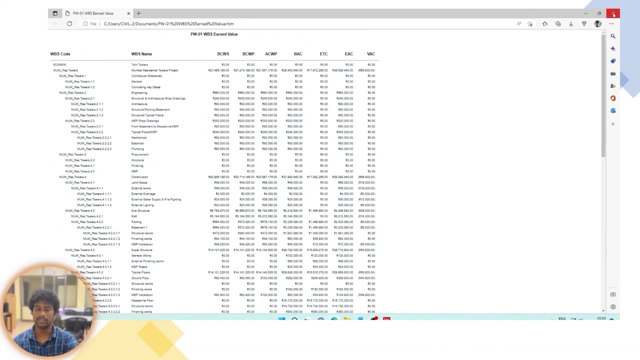 These are the standard reports. It is available for every project in a primary basic software. So these templates, basically it's designed by the organization, policies and everything to maintain standard policies, standard documents, So, and these are maintained and managed for every project within this, for every project. 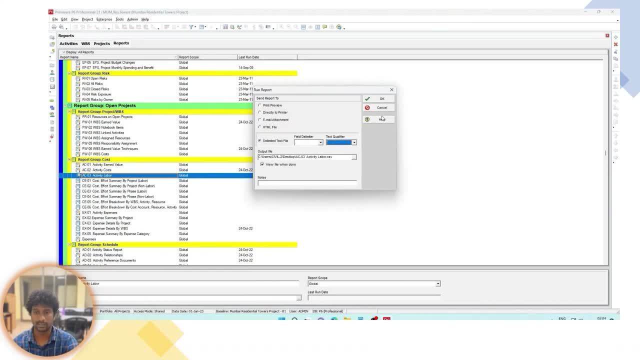 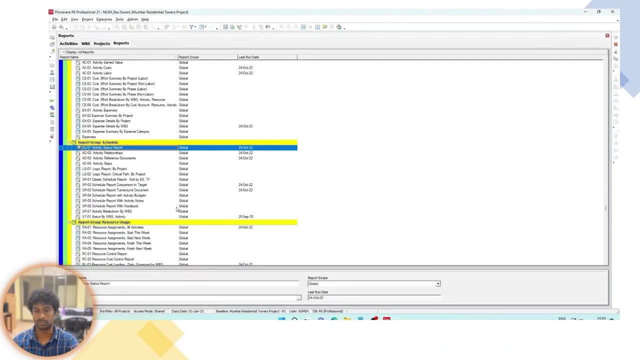 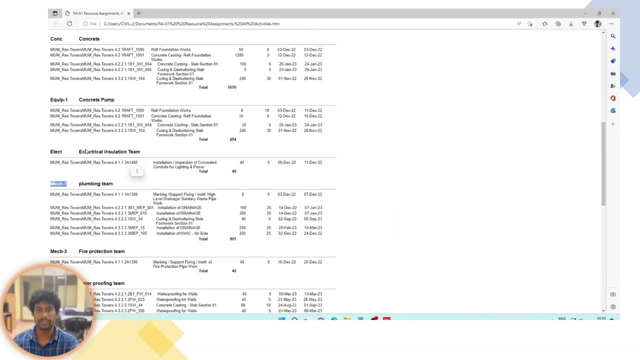 So these are dedicated report. There is in a dedicated report section primary software. from that you can produce 50 plus standard or batch reports. It's related to the scheduling, it's related to the reports for monitoring and everything Also. you can modify those. 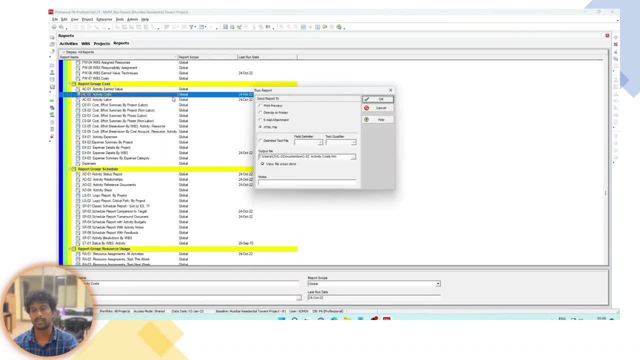 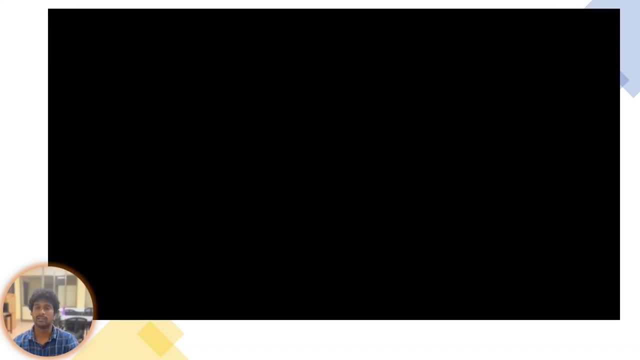 Those reports can save it further use, like you can save, as a templates. If you've done all these printing final reports, the next step is integrating with the tools. This is the advanced step in Primavera. Primavera has given a feasibility to connect other tools like business intelligence data. 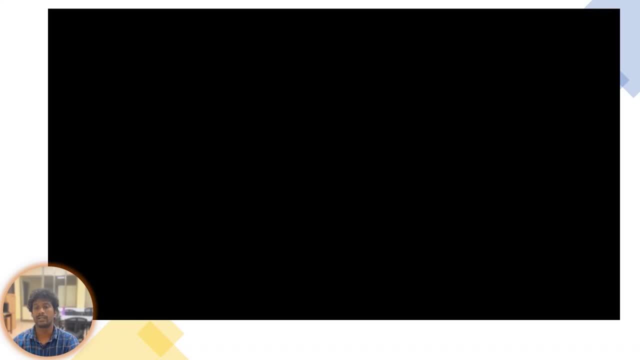 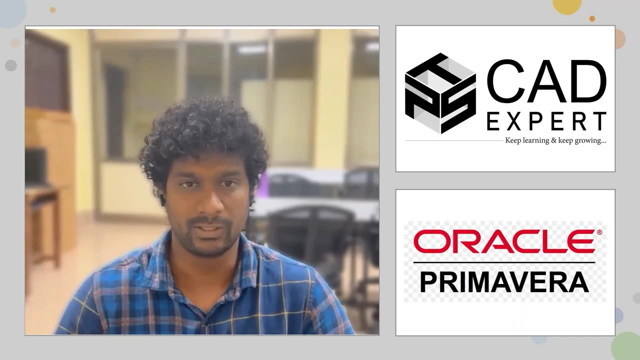 visualization and risk analysis tools, And this step is dedicated to explore all possible ways of integration. I hope you understand all the steps. in a place like Primavera, The question is: is it required to execute all these steps for every planned project? 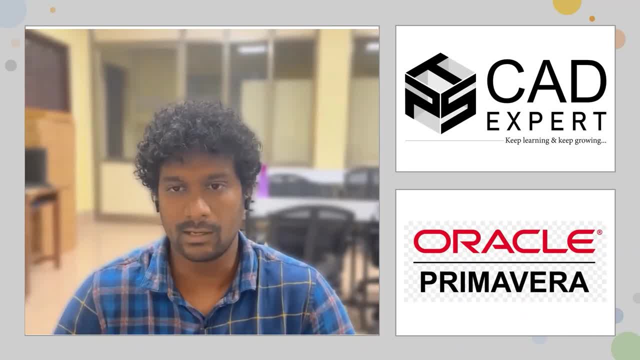 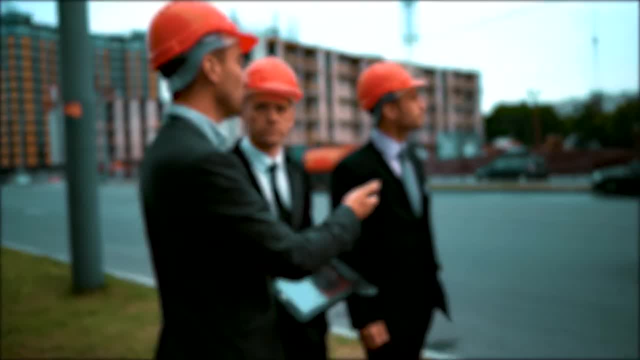 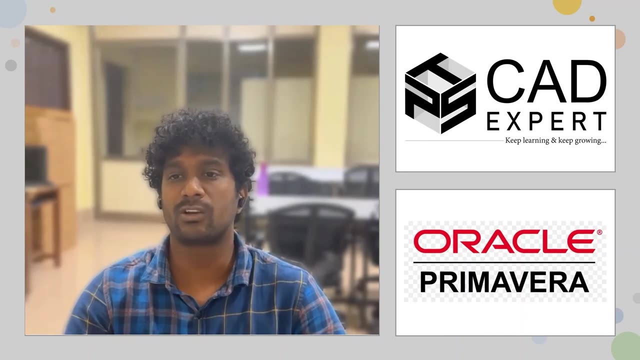 Answer is maybe no. You know why. In a practical planning of a project, there are only two approaches. One is for like: are you planning for estimation? Are you planning for the control? So what is the difference between them? Planning for estimation approach: the objective is to create a schedule with the cost that. 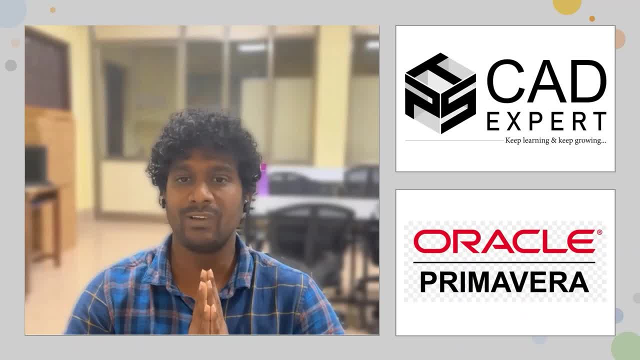 are used only as an estimate. The schedule will never be updated. Activities may have many resources assigned to them or to develop an accurate cost estimate, and include many items that would never be updated during the process of updating a schedule. Here, my intentions are clear. 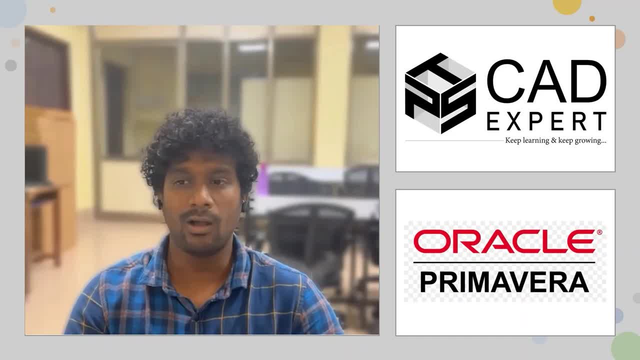 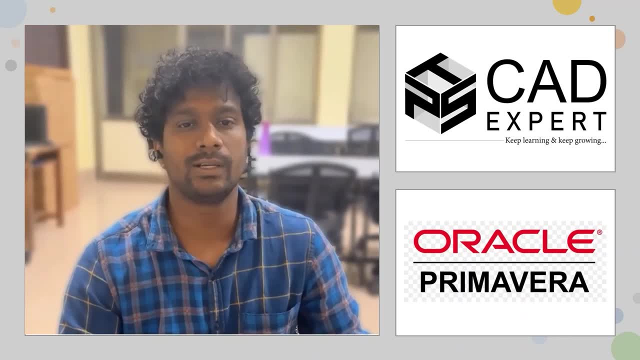 I will use my planning for a budget estimation. I add all resources that are involved Planning for control approach. In this approach, my objective is to control and monitor the resource units that are assigned to activities. I will keep on updating them. I will use the actual units used during the project execution. 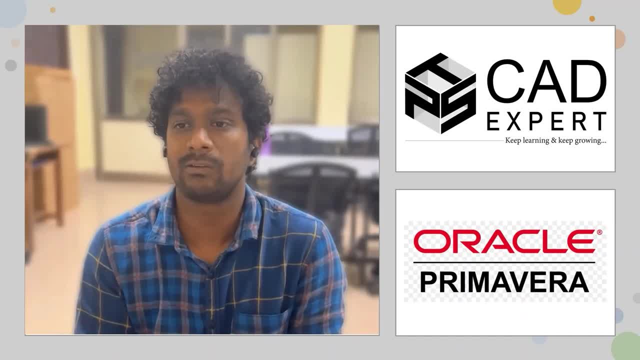 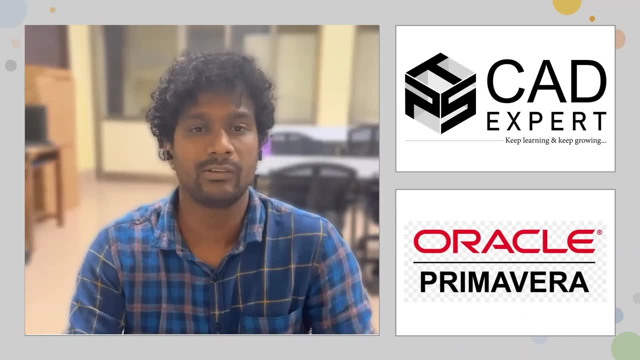 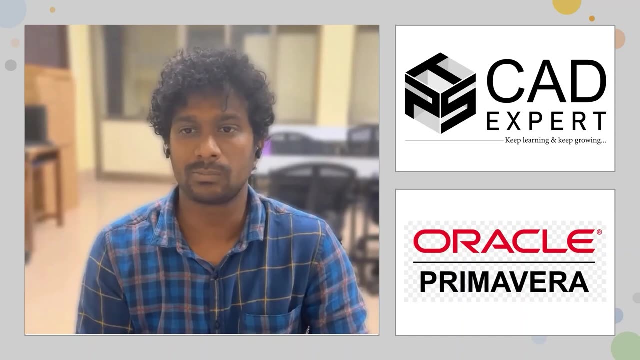 Possibly, I will perform n-value analysis to understand the deviance between the planned versus actual. So in this it is important to ensure that the minimum number of resources are assigned to activities, and preferably only one or two resources assigned to each activity. When a schedule has many resources per activity, the process of updating a schedule becomes. 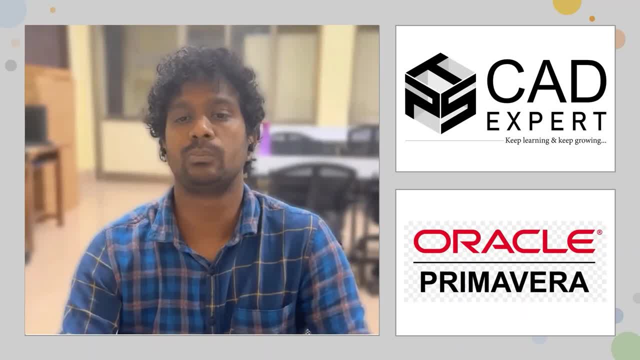 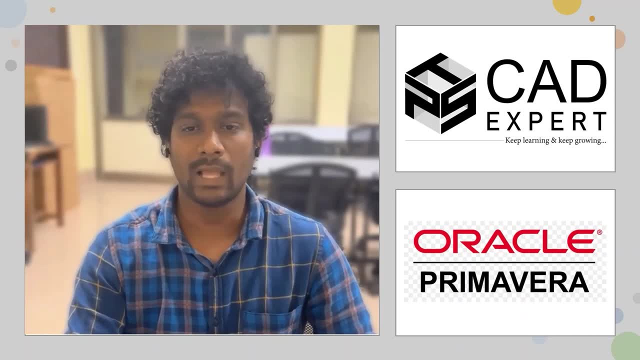 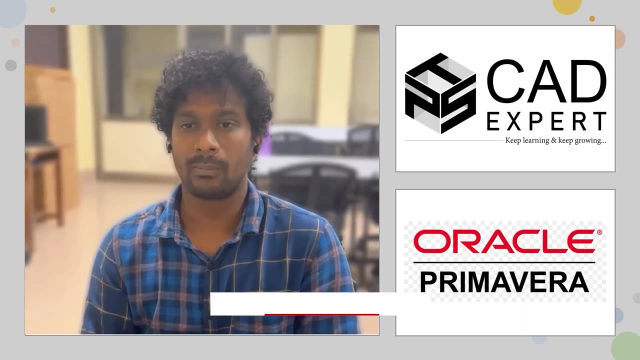 extremely difficult and time consuming. So balance should be there between the number of activities and the number of resources. Maintain single rule: like more activities have a schedule has, the less resource should be created and assigned to the activities For more contents related to the Primavera. please like and subscribe this channel and.